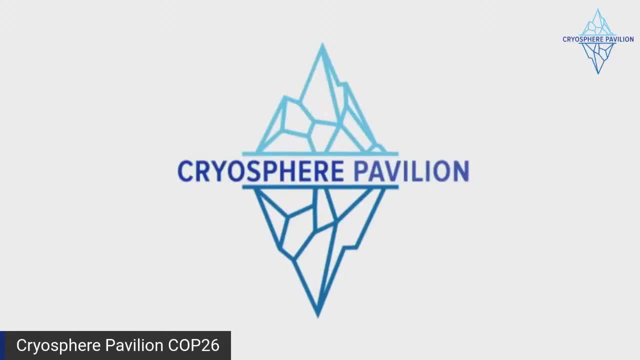 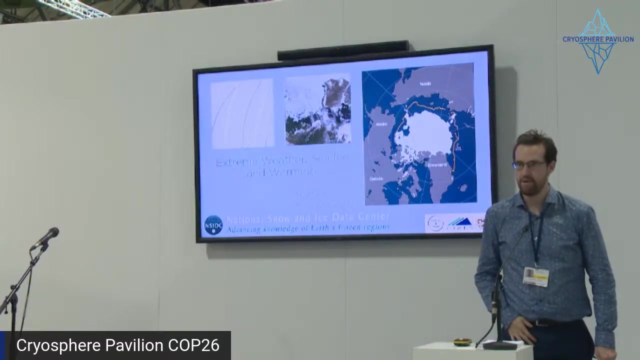 We have our little ice bath over here. Thank you, Hello and welcome. My name is Tom Webb. I am a postdoctoral researcher at the University of York studying the coastal cryosphere. Welcome to the Cryosphere Pavilion and this session on extreme weather, sea ice and Arctic warming. 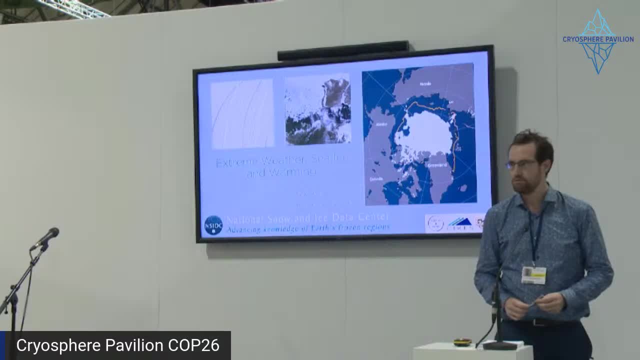 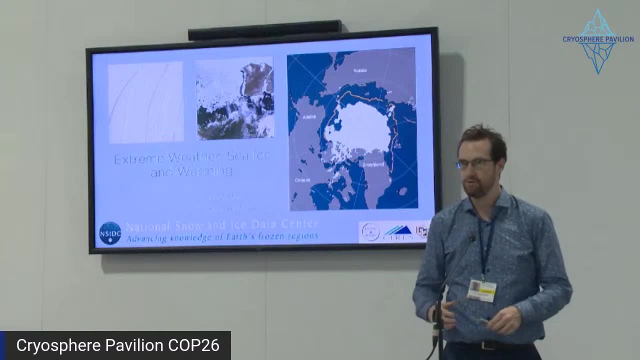 We are joined by hubs in Geneva and also in Stockholm. If you have any questions, feel free to ask us in the chat or at your hubs directed to us. We will also be talking to the speaker in the question and answer session. So now let me welcome Walt Meyer to the stage. 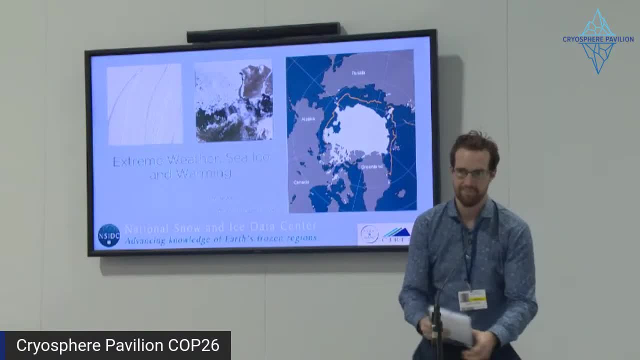 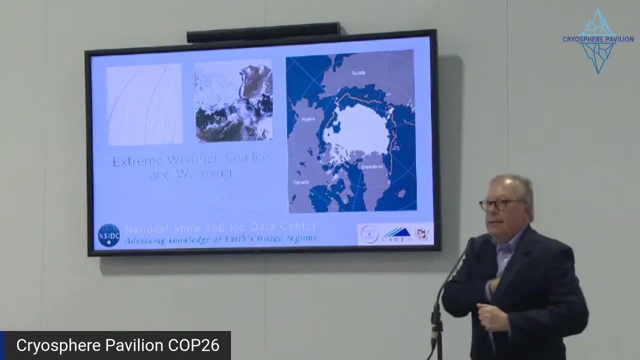 He is from the University of Colorado, Boulder, and also the National Snow and Ice Data Center. Thank you All right, Thank you for the introduction. We will talk a little bit. This will be fairly short, A little bit about sea ice and the warming and some of the impacts on extremes that we see both within and potentially outside of the Arctic as well. 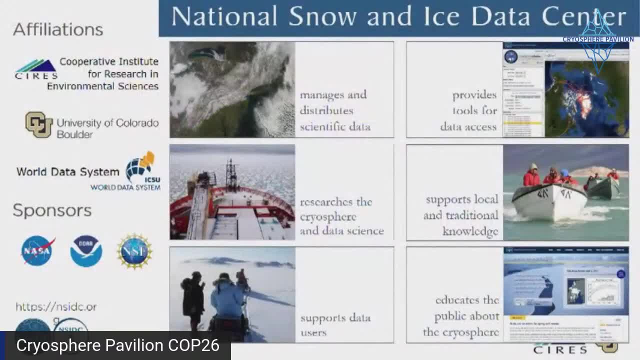 So I am at the National Snow and Ice Data Center and we are at the University of Colorado. And just a quick little background for folks that are not familiar: We have a pretty sizable research group and do a lot of research in all kinds of aspects of the cryosphere. 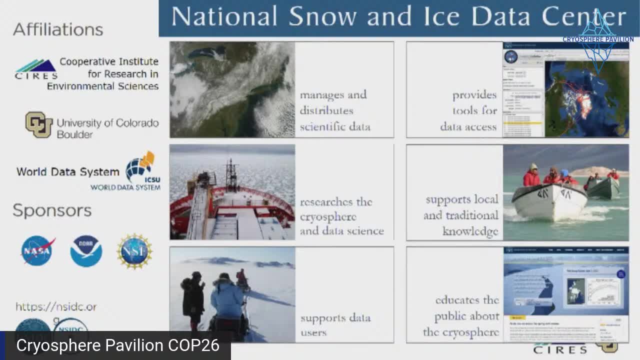 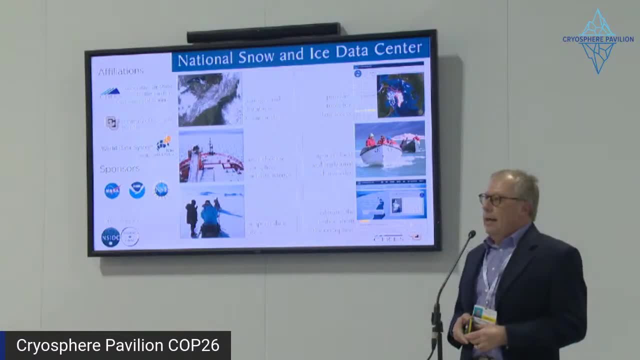 Snow, sea, ice, permafrost, glaciers, Greenland, Antarctica. But our main part, our main section, is actually on data archive and distribution. We are one of the NASA main NASA data centers, for the data center for snow and ice, So we archive all the NASA products. 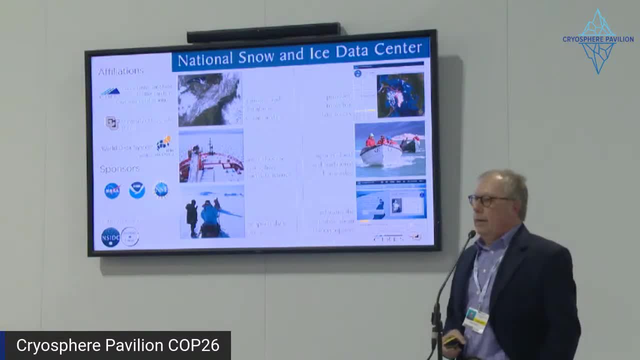 We also have a NOAA data center there as well, And how is that? We also have some projects that support local research, That support local and traditional knowledge, So that is also a component. We do research with communities and partner with communities in the Arctic. 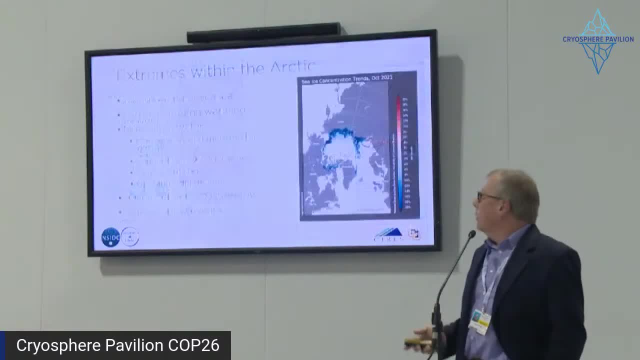 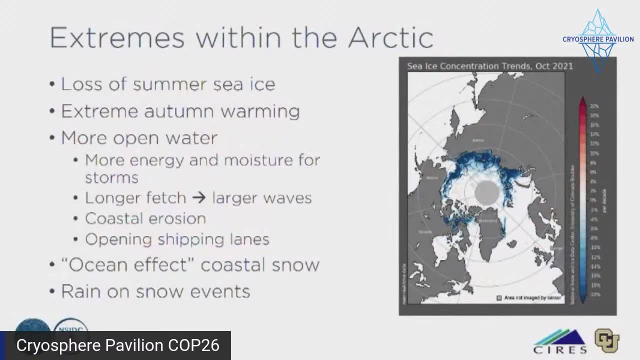 And do some outreach in public education as well. So, in terms of the Arctic- for those that were at my previous presentation, I talked about the extremes that we are seeing in the Arctic. You are probably familiar with the real extreme sea ice loss that we have seen. 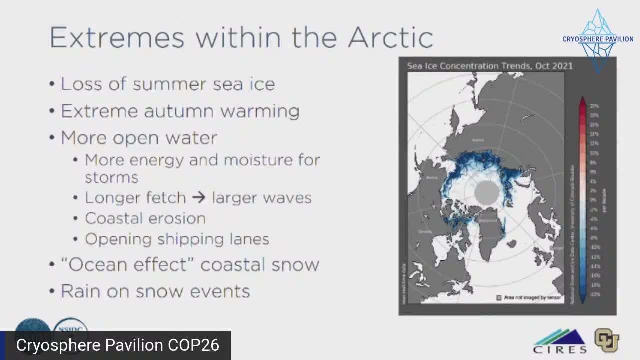 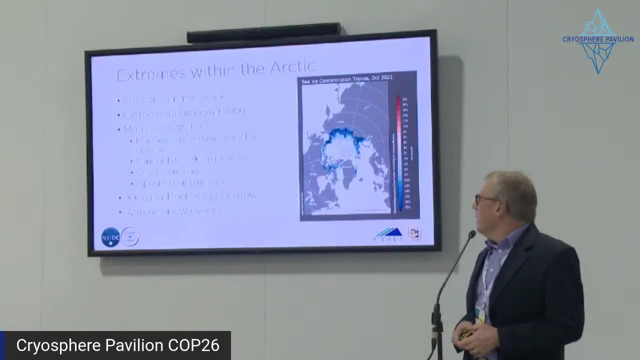 That is one of the big changes in terms of the Arctic, In terms of the Arctic Ocean. There is much less ice cover year round, Particularly during the summer season and into the autumn, And this is one of the- this is the October trend. 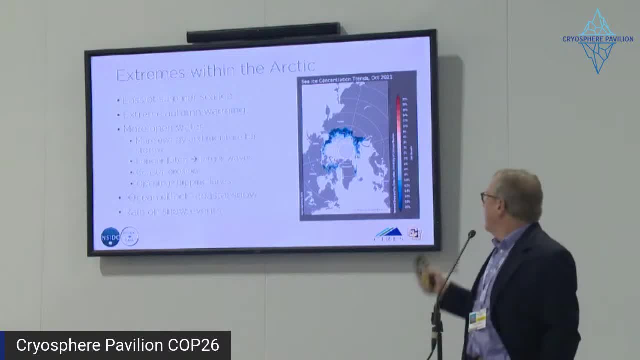 You can see the significant trend in the blue shades there- About 12-13% per decade- of losing ice, Particularly on the Siberian side, And that leads to more autumn warming. One of the things, One of the biggest signals we see in the Arctic in terms of the climate is the warming in the autumn. 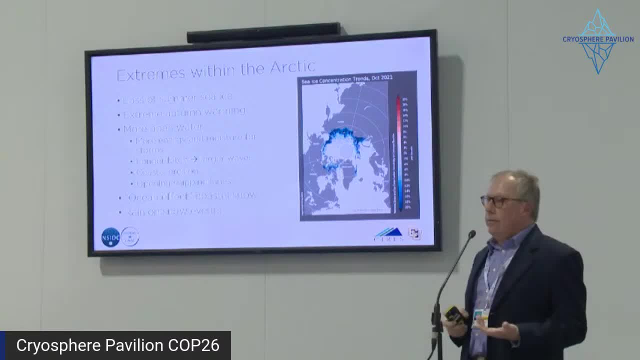 Because what happens is you have the ice free ocean in October, into November And even into December now, And the atmosphere- The sun has gone down, The atmosphere starts to cool, But you have this big heat source And that heat is providing energy and providing heat to the Arctic. 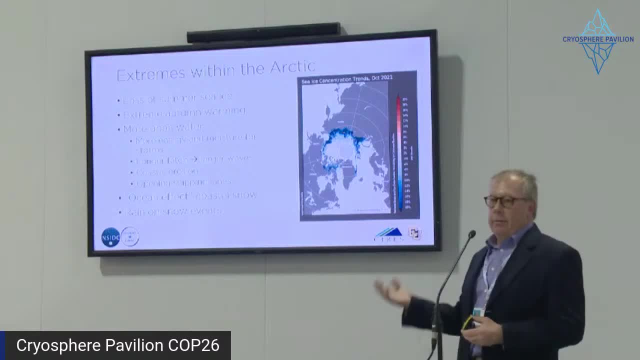 And keeps the atmosphere warmer. So you see a lot of surface level And even that heat even goes up higher into the atmosphere. So that autumn warming, That open water, It's more energy and more moisture, So potential for greater, more storms. 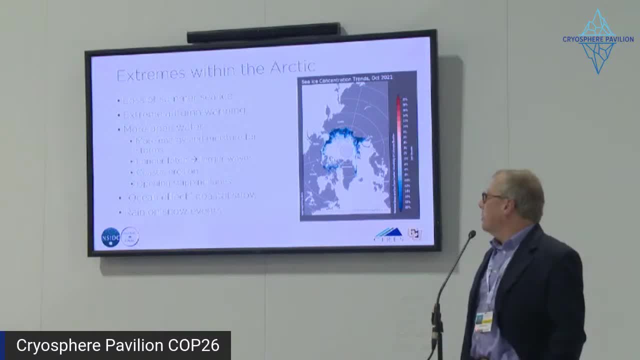 And greater, more significant storms. There's also more open water. This is throughout the summer, even, And even you know you have earlier opening in the springtime, So you overall have more open water. It's a longer fetch area of open water where the winds can blow across. 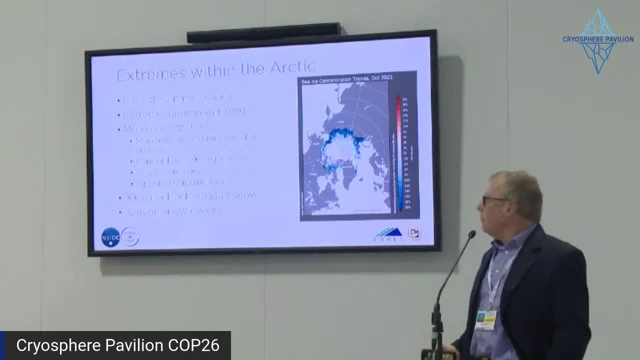 So that leads to larger waves And the coastline. those can have big impacts: Coastal flooding And then, as we're also seeing, thawing and permafrost along the coastline and throughout the Arctic. That leads to coastal erosion And, as we're opening things up, there's also an impact in terms of open shipping lanes. 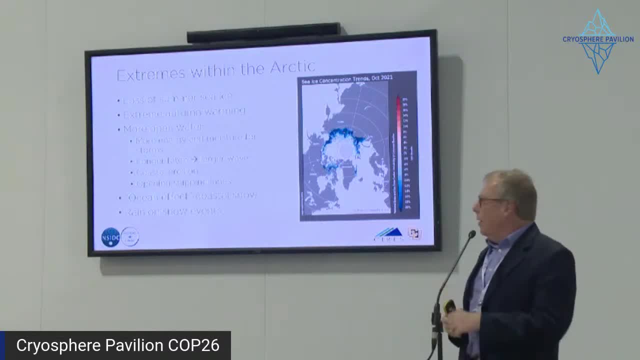 And then the ocean effect, Coastal snow, which I'll talk about in a minute- We'll talk about it in a couple minutes too- And rain. on snow events, I'm not going to talk too much about that. There's a group at NSIDC- where I'm at- that has a project that is looking at this. 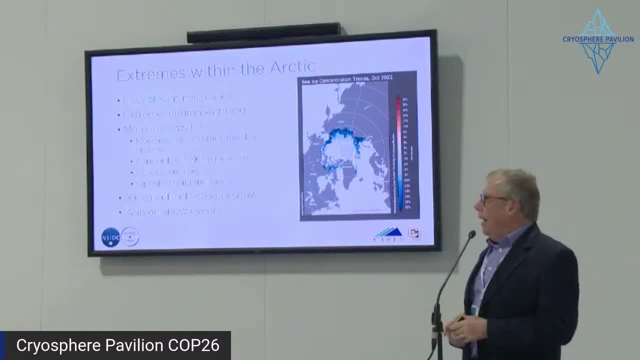 Led by my colleague, our director Mark Ceres, And these have a big impact as well. Where you're getting warmer temperatures, You have more rain events instead of snow events, And that rain on snow has big impacts on the terrestrial As well as, potentially, on the ocean. 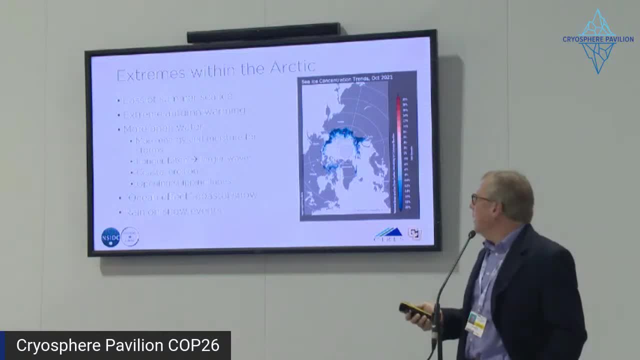 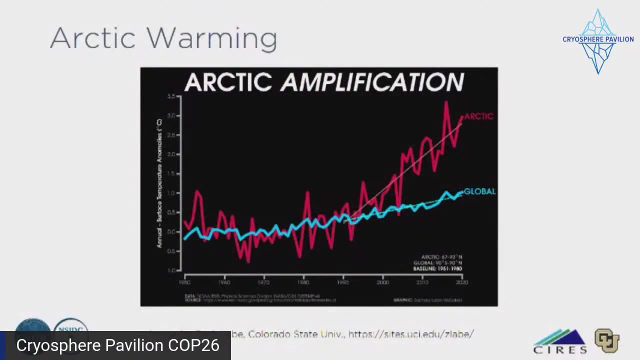 On the sea, ice and ocean areas. So folks have probably seen this. The Arctic amplification: This is where the Arctic is warming two to three times faster than the rest of the globe. This is a really nice image, Zach Laib, who's at Colorado State University. 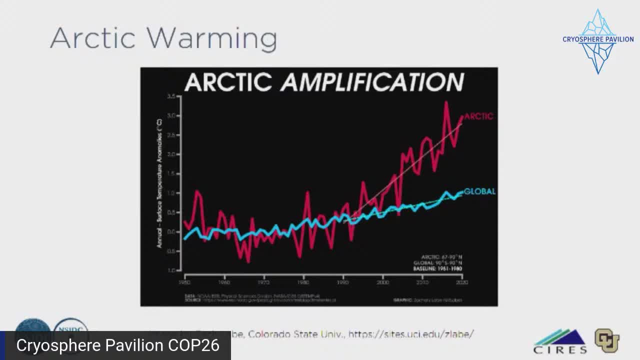 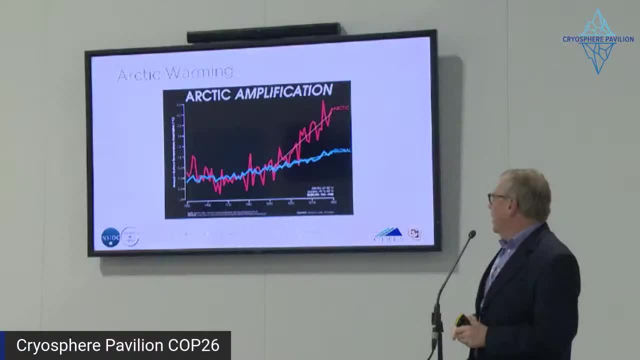 He has a really nice website and puts together some really nice figures. So I often steal liberally from him Because it saves me a lot of time. But this is a really nice figure. This is from NOAA and NASA GISS temperatures And you see the Arctic is about a three degree temperature. Three degree C temperature increase, compared to about a degree for the global average, And this is due to the loss of sea ice and the feedbacks that we see As the Arctic sea ice decreases. You've got the high albedo sea ice being replaced by the low albedo ocean. 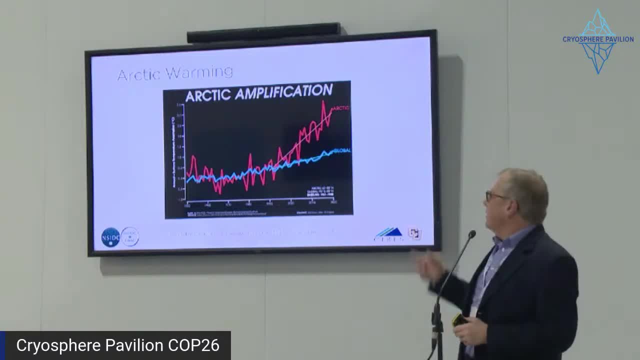 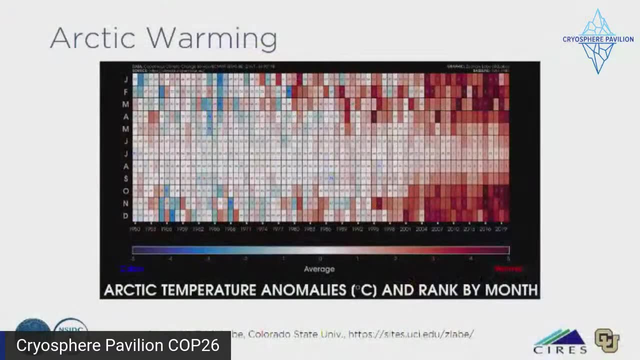 That means more heat gets absorbed And again, a lot of this is happening in the autumn And into winter region. And this next shows that this is a little complicated. But this is another nice figure from Zach Laib: January through December on the Y axis, from top to bottom. 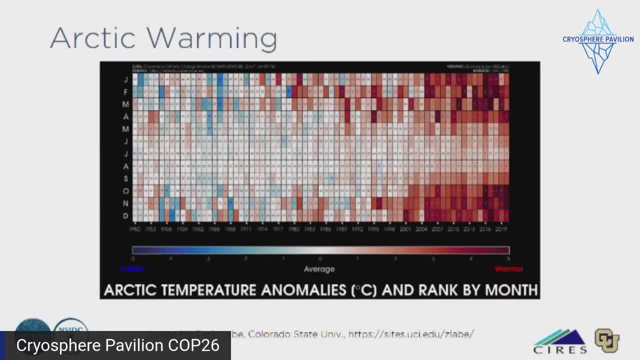 And then the years on the X axis, starting in 1950 actually, And this is basically the ranking of the individual years for each month, And basically the colder months, the lower ranked years are in blue And then it converts into red. It converts into red for the warmest. 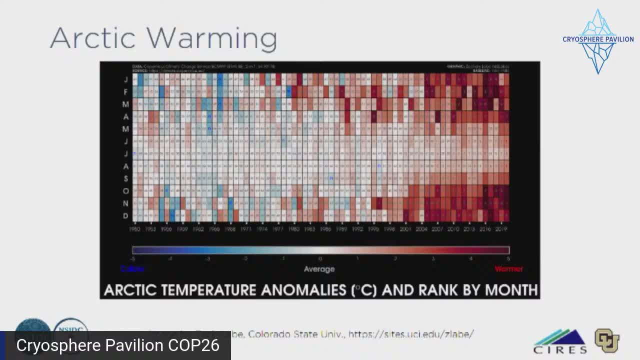 So the darkest red is the warmest year of each month, And then the darkest blue is the coldest year, And what you see? obviously all the red is over on the right side in the more recent years. So this is year warming. 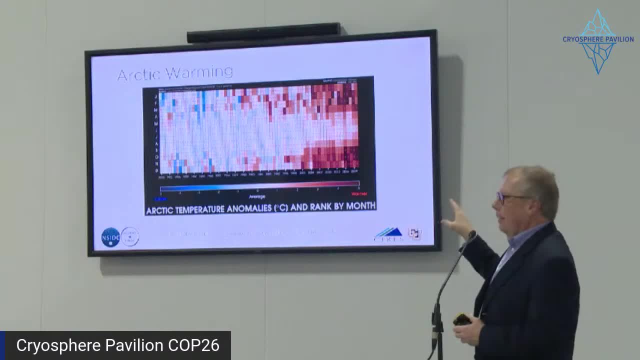 But you also see, the red is focused on the autumn, into winter And to some degree into spring, March and April as well, Not so much in the summer, And that's because you have in the summertime all the energy is going into melting the ice. So there's not as much of an anomaly in the temperature, Even though you have a lot more energy going into the system. you're melting the ice or you're warming the ocean, And the atmosphere stays pretty much the same. So it's less. there's still a warming trend, but it's much less notable than in the autumn and through spring. 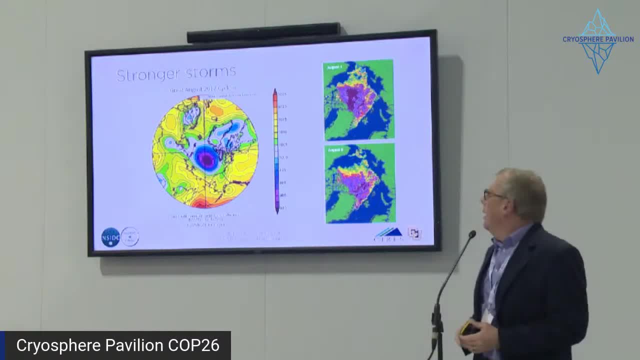 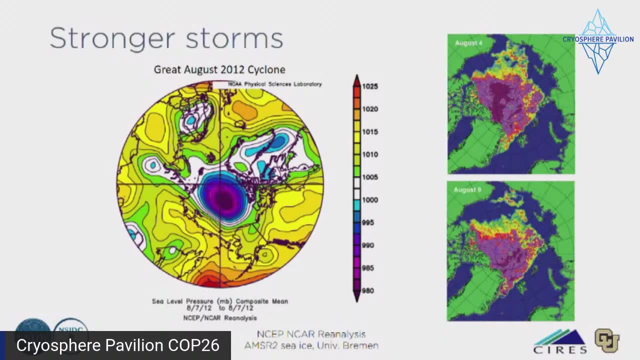 So stronger storms, One of the you know you have the ocean And that provides a source for humidity, for moisture and heat for storms. So when you have ice not present, that allows these storms that can develop and then penetrate farther into the ice pack and into the Arctic in general. 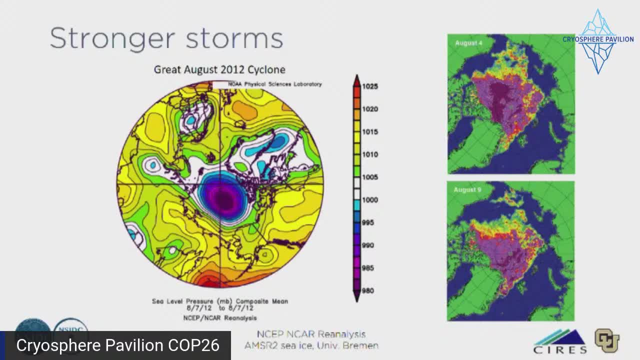 And one of the most notable ones that we had was what we call the greenhouse, The Great August Cyclone in 2012.. That was a really strong low- below 980 millibar low, So very strong- And it tracked into the Arctic. 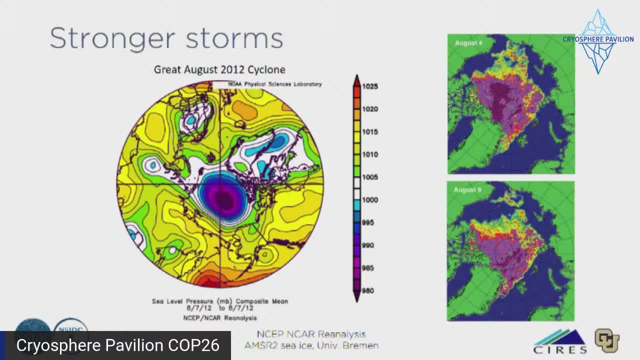 And one of the things that was notable for at that time was what it did to the sea ice. It tracked in the top is: this is University of Bremen sea ice. the concentration Purple is the highest concentration. I left off a color scale there. 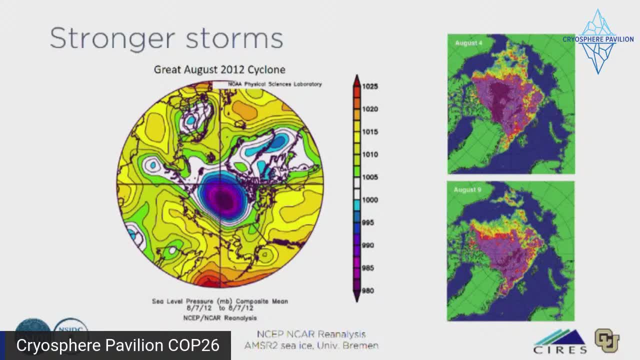 And you see a bunch of ice in, like the Beaufort Chukchi East Siberian Sea region there on August 4th And less than a week later, five days later, most of that ice had disappeared And that's where this cyclone turned across. And basically it brought heat. It turned the waves, It really it mixed up. ocean heat Brought in atmospheric heat. The waves broke up the ice cover And really caused the ice to really the ice loss to really accelerate. So this was one factor in why the 2012 storm. 2012 is our record low sea ice rate And it still is, Because of that storm, Not the only reason. It was a really warm year And we had a lot of ice melt anyway, But that was a big factor And one of the things with that. you know, it hit at the right place and at the right time. 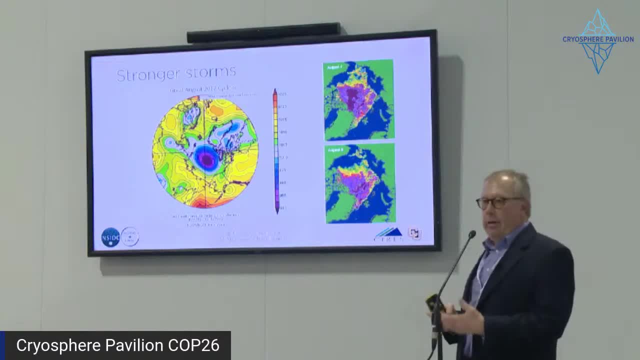 August. August is normally a period when things are starting to freeze up. in the high north You still are melting ice in the around the ice edge. That's mainly due to the ocean heat. actually, at that point, By the time you get to August, 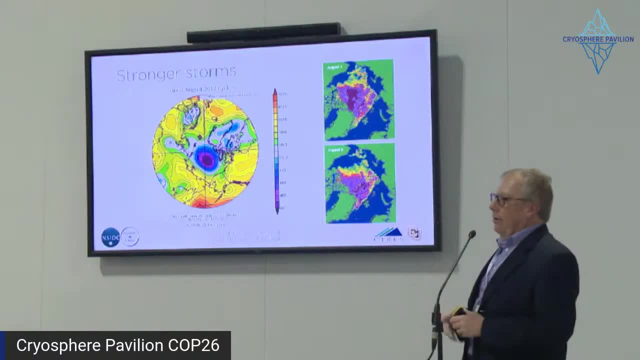 The sun is going down, But this was actually. we saw an acceleration in the ice loss in August, So that was really unusual. We haven't seen quite the same thing since then, And that's because we have had storms come through, And some pretty strong ones. 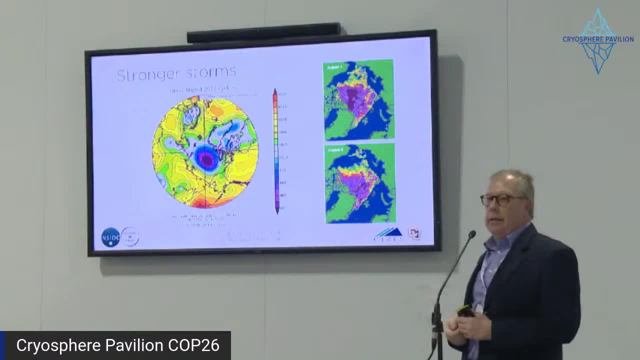 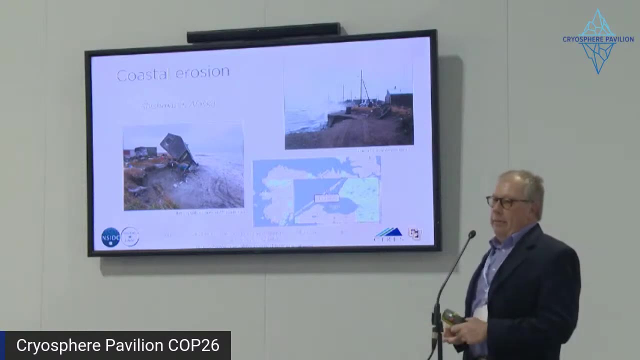 But they haven't tracked in the right place, in the right direction To cause the rapid ice loss. But what we do see happen Is if these storms track over open water towards the coastline, Then you have potential impacts And again it depends where they track. 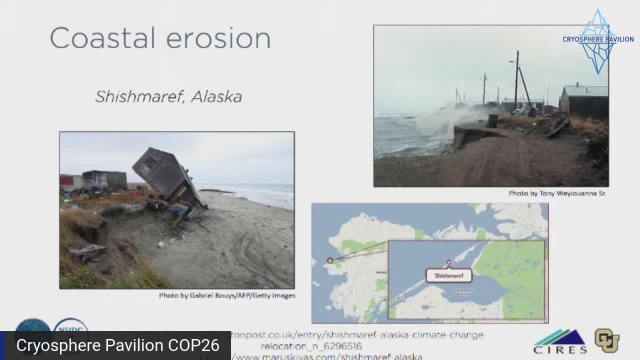 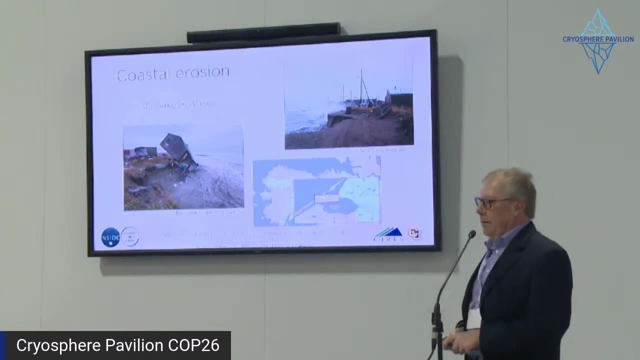 And when, But there's been several cases of some pretty extreme coastal erosion With these northern communities along the coast. The most famous one is Shishmaref, Alaska, And it's gotten a lot of notice. You probably have heard about it. 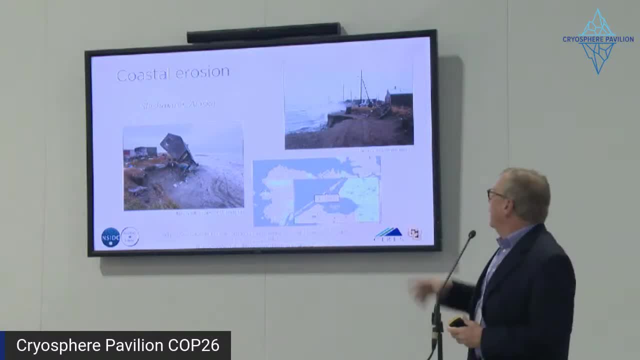 Because they actually have. They've started to lose buildings, Roads have been washed away. It's right on the coast, It's on a little spit of land of island there, Right on the coast, And it's built mostly on soil above permafrost. 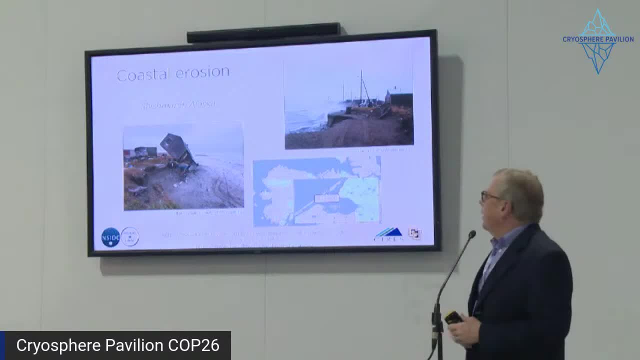 And the permafrost is thawing. So you have that collapsing soil And they've actually started to move buildings inland Back over to the mainland. even Because of this, Because they're going to, They're potentially going to lose the whole town. 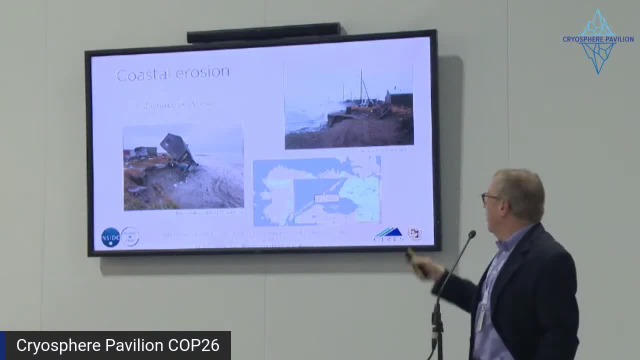 At some point, And there's other villages, Like Kivalina is another one Which is, I think, on the other side of the bay there, That are losing Moving coastline. So, And these are, You know, One of the main factors again. 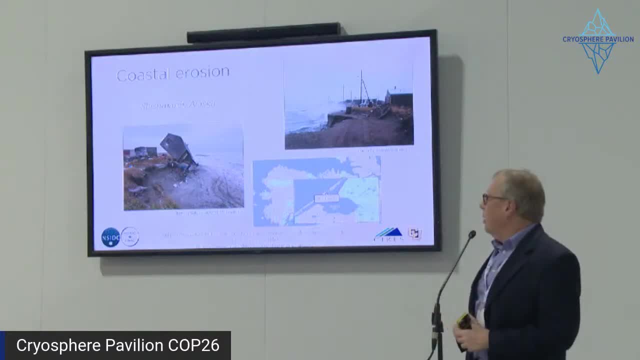 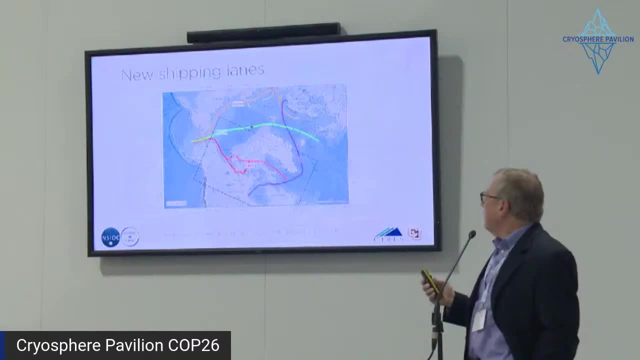 Is you have the increased fetch, The waves, Especially when you have storms And the permafrost is thawing, And so you can really lose coastline very quickly. Another aspect that kind of relates back to the issues In the last session. 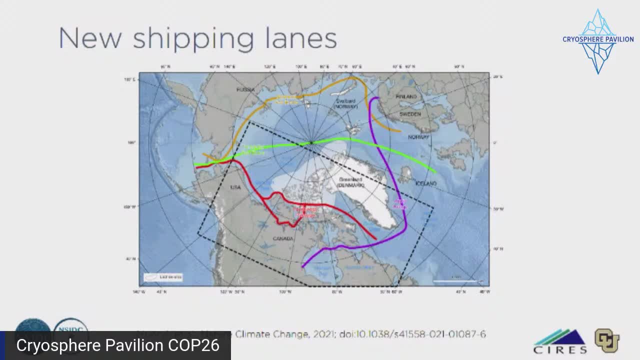 And concerns in the last session. As we open up the ice cover, You know We are opening up shipping lanes. You know, Particularly the northern sea route Is Has been largely open, And then the Transpolar sea route over the pole. 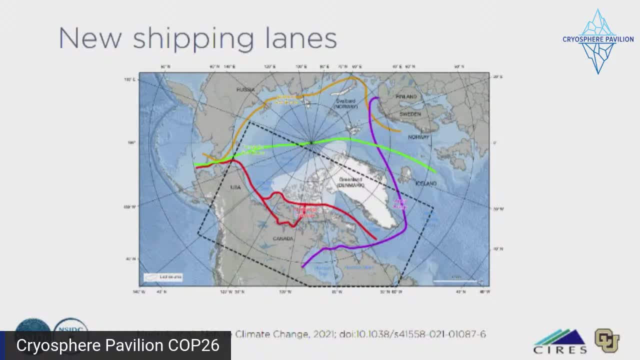 Is potentially, You know, A real shortcut And would be largely through- You know Completely- international waters. And then there's the northwest passage, Which still has a lot of issues And will continue Because of the- You know The. 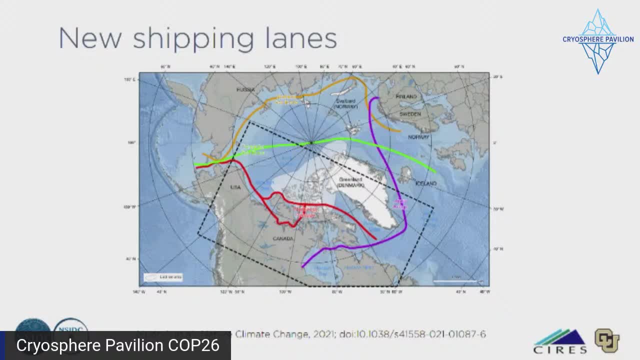 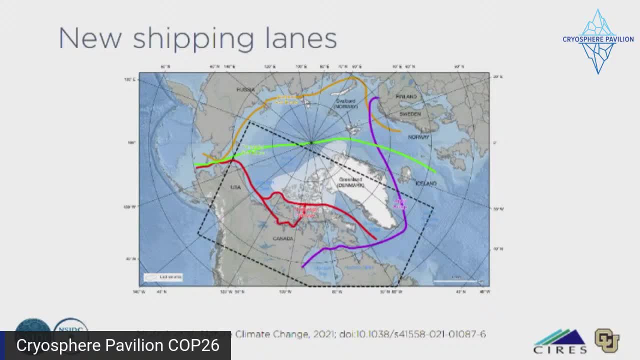 And more of them There is. There is a lot of risk with greater storms As well as the remaining ice cover. This is A paper recently by Lawrence Mudric And others. You know iye on the American side In 2014.. 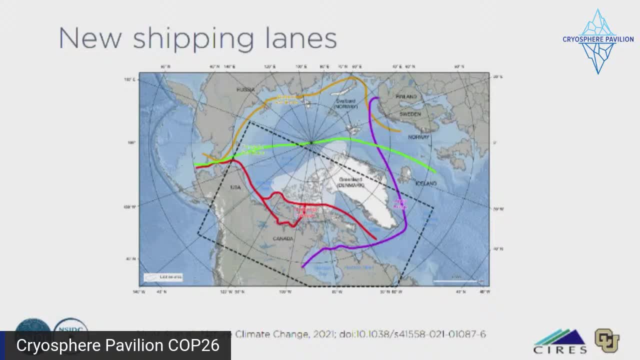 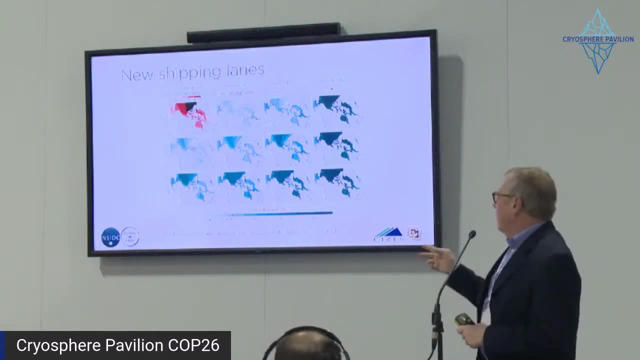 Where What happened. So the major investment Was when the marshals brought in redesigned quello mixing. Alright, That's where we are today at the moment faculty. All right, Thank you very much. Thank you, willen. Environment Canada. that showed how the change in season is going to increase under different 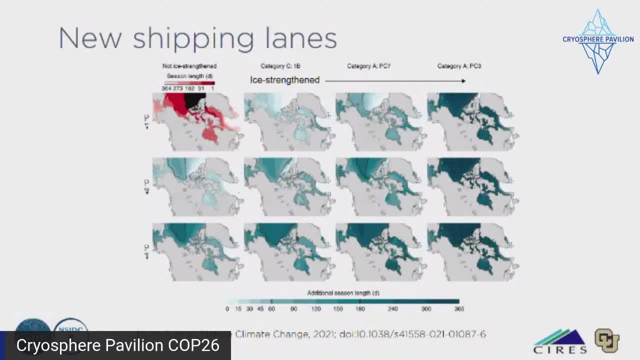 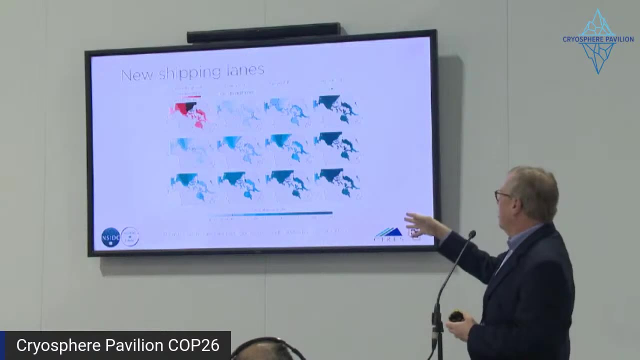 scenarios. So the top line is the one degree. That's basically where we're at, And the not ice strengthened is on the left column, And then the three on the right are ice strengthened at various strengths, So the weakest to the largest or most strongest, And then the blue shades are. 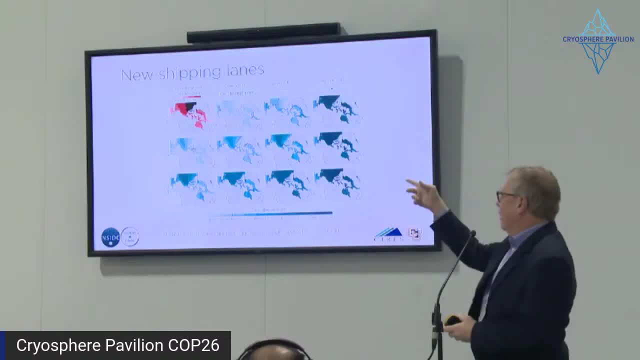 the additional strength over what you get from the current, not ice strengthened, And you basically see, as you expect, plus two degrees. you significantly lengthen the ice season or ice free season where they can transit, or the time they can transit, either through ice free conditions. 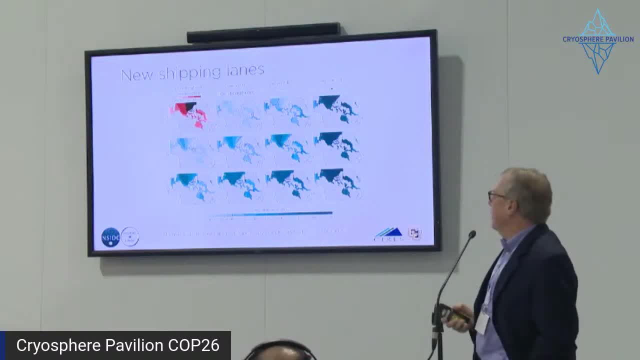 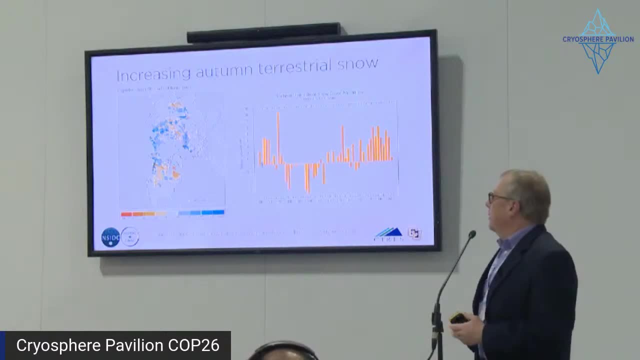 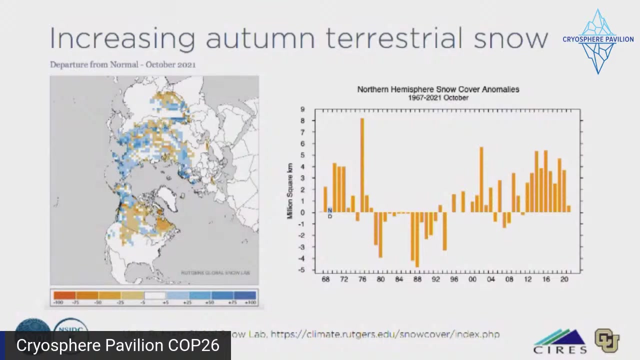 or lower ice conditions where the less strength and ships can go. The other thing that I mentioned- that is an interesting effect as well- is the potential for increasing terrestrial snow cover. When you have a big area of open water, you have the cooling atmosphere in the autumn. What happens when you have ocean? 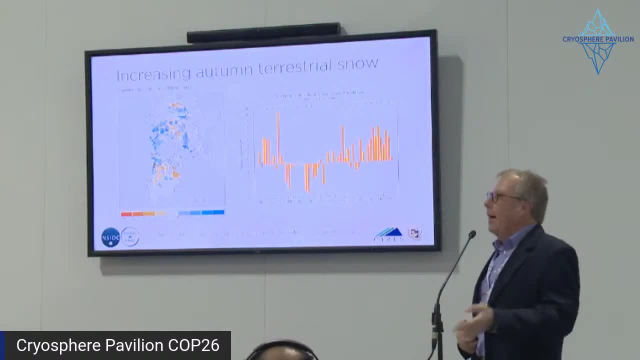 warm, moist ocean going across. wind blowing from that onto the cold land you can get coastal snow. I grew up in Michigan And that was a very common thing in Michigan. in the Midwest You get the lake effect, what they call the lake effect snow where the lakes haven't frozen up yet. You get the winds blow from the west. 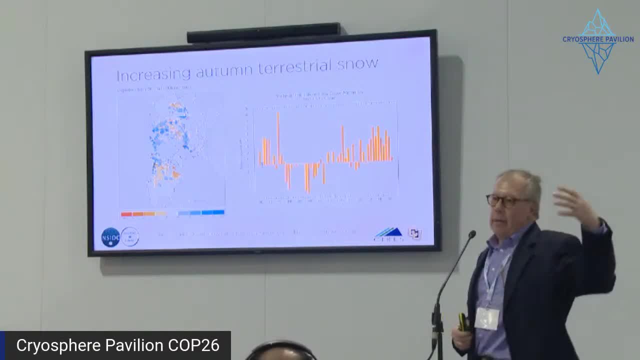 or from the south or north, and you get cold air comes across, picks up all the moisture in the in the heat from the lake, hits the land in that cold air and it just dumps all snow. So you know, I have sisters actually live right on the coast of the state of Michigan and they live in the. 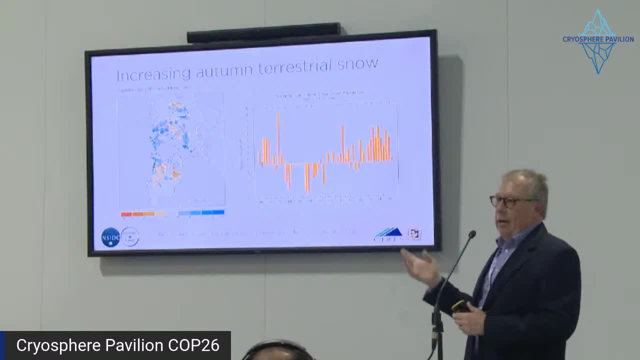 lake, michigan, and, uh, you know you'd be, you know, 100 kilometers away, and it'd be nice and sunny and clear. and then you get to the coastline and be, it'd be in the middle of a blizzard and you get the same effect from the oceans? um, you can, because, again, depending on where the 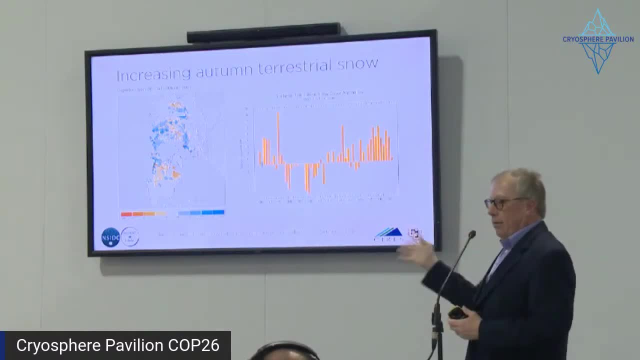 where the circulation is. you can get um going across the open ocean in the autumn, over the land, particularly in siberia, as well as in places in alaska, and we see this is in october. this is from the rutgers global snow lab where they're mapping the the overall snow extent and anomalies um so. 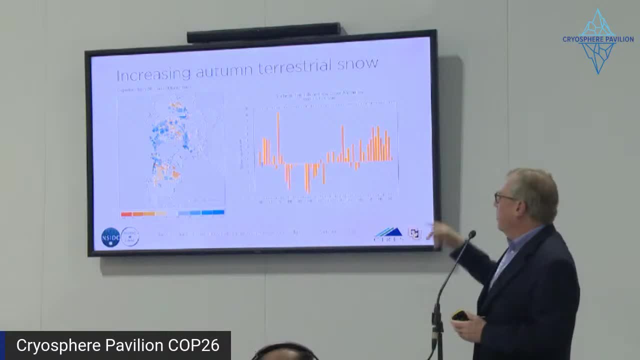 this is the uh anomaly of the total extent in october and you can actually see there is a pretty clear increasing trend uh over the last 20 plus years or so, 25 years or so. so this is in some ways it might seem counterintuitive. we think of you know warming um snow is should be decreasing you. 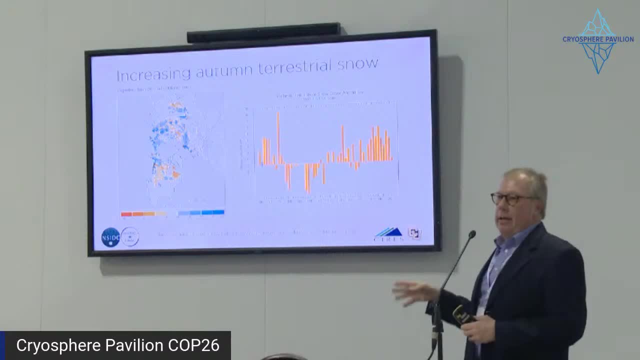 know that ice is decreasing, snow is decreasing. it's definitely true that snow is decreasing in springtime. we're seeing much earlier melts in springtime, but in the autumn, at least in some areas, we're seeing increases, particularly in the arctic regions, and that is at least partly due to. 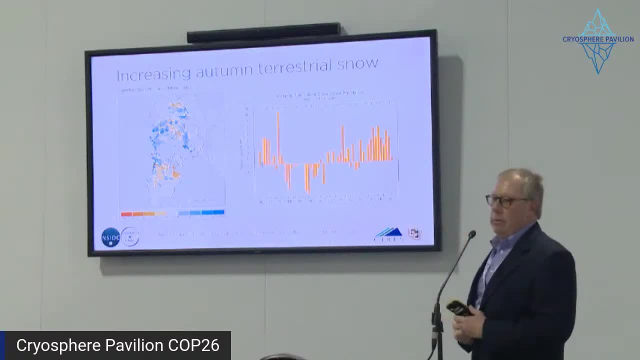 the uh, this effect of having this open water source available as the land is cooling and the ocean remains warmer. and uh, october's november looks very similar to this. i just chose october because it's the most recent data. this is actually uh. on the left is october 2021 and you actually do. 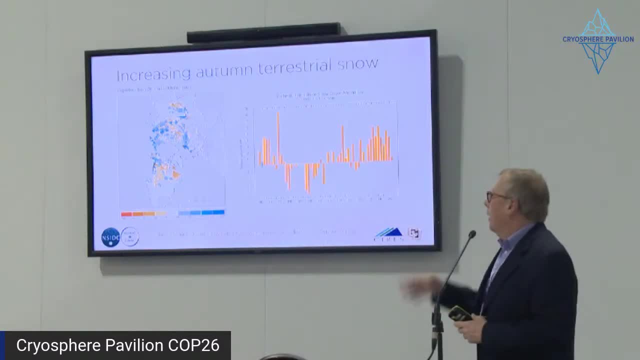 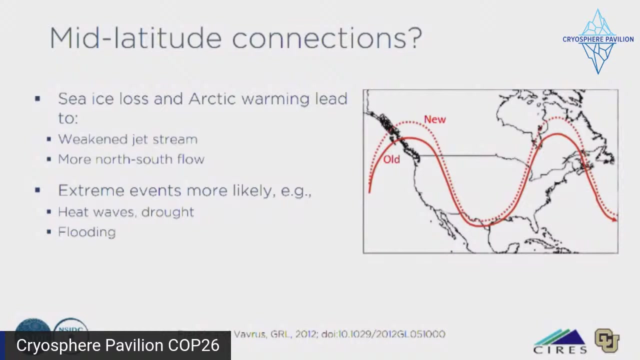 have a 50 to 50 or so increase snow cover. um, that's just one month, but the trend on the right shows you that there there is a a definite, uh, increasing trend there. um, so that's kind of the impacts of the extremes in the in the arctic region. um, probably not comprehensive, um, but that's. 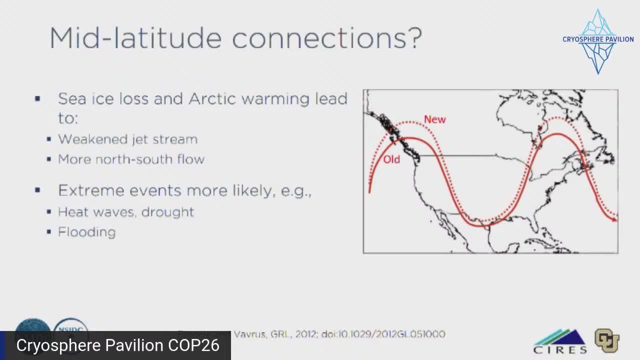 kind of just a quick uh summary of those, the other extremes that people talk about a lot is the mid-latitude connection, the connection between the arctic region and the arctic region, connection between the arctic and the changes in in the sea ice and the arctic. warming um and and 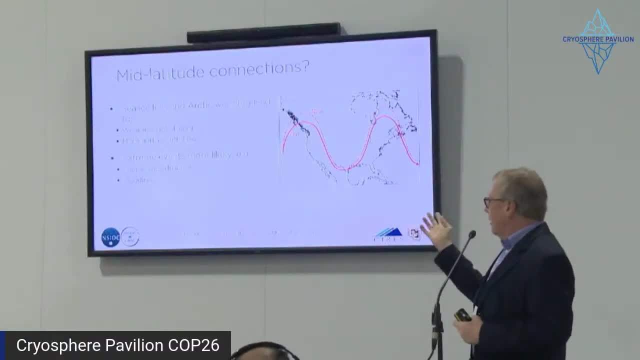 how that may affect the mid-latitudes, and this was a really big paper uh, jennifer francis and steve babris uh, in geophysical research letters published in 2012, and this in in our community. i'd say this made a bang. this was, you know, maybe not quite einstein special relativity level, um, but 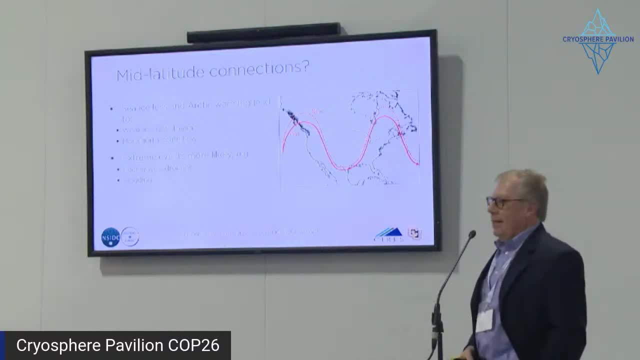 this was a pretty big paper, um, and really got a lot of attention. and it got a lot of attention, uh, in, in, in, in many ways, um. so the first to kind of just quickly summarize their paper. the idea is: you, you're, you're warming the arctic and you're, you're. 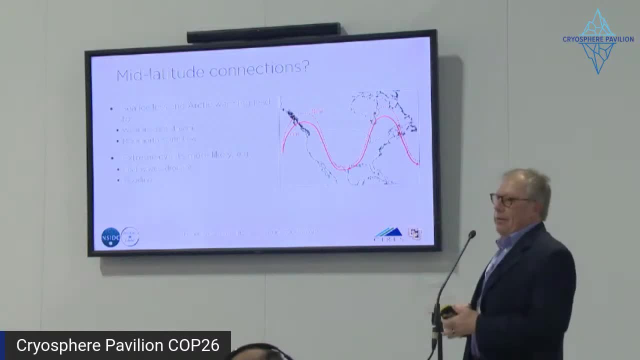 losing sea ice, you're warming the arctic, that's, that's changing the balance between the warm art or the cold arctic and the warmer mid-latitudes, and the jet stream kind of, is essentially set up by this balance, by the, the colder arctic and the warmer mid-latitude, and you can 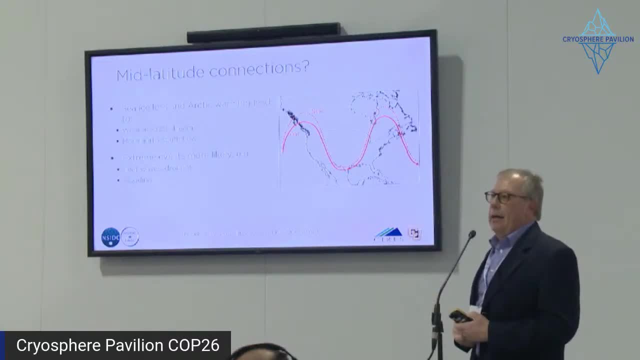 break down. that can break down from time to time, uh, as cold air spills out, um, and the jet stream gets kind of wavy instead of being more west to east flow, and the idea is, is that as you warm the arctic, that balance is, it's decreasing, so it's more easy for that, that outflow of that colder. 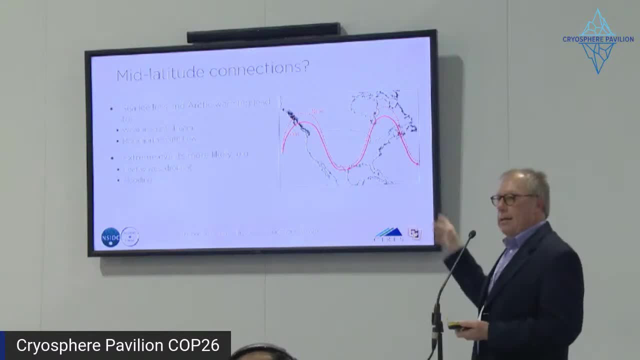 air, which is relatively less cold, to spill out and cause this wavy jet stream, and that that does is more south flow instead of a east, instead of a west to east flow. um, and that can that leads to, uh, more extreme events. so, when you have this wavier jet stream that allows, you know, air from the south, 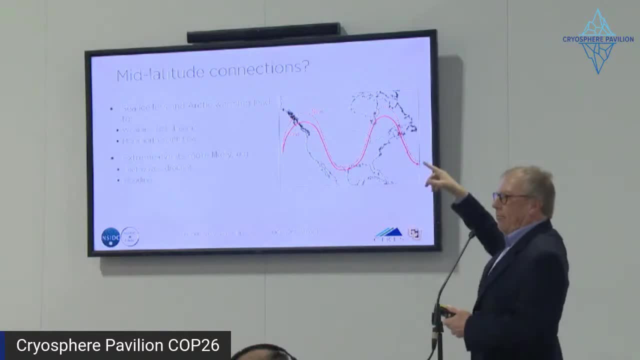 to more easily infiltrate north on the one side, or from the south, or from the north to filter eight south so you can get cold air outbreaks, you can get heat waves um you also. it also tends to slow storm tracks so you get more extreme events like uh. 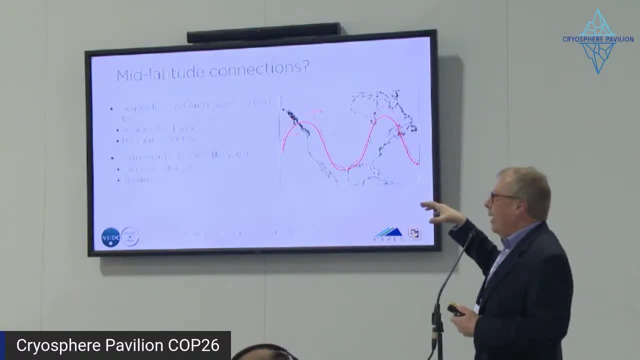 you know, you get highs that get stuck and you get a heat wave and drought. um, you can get flooding, you get a storm that moves very slowly as the, the jet stream doesn't move it out like it normally would. um, so that's kind of the idea behind the uh, behind that paper and behind the idea of this. 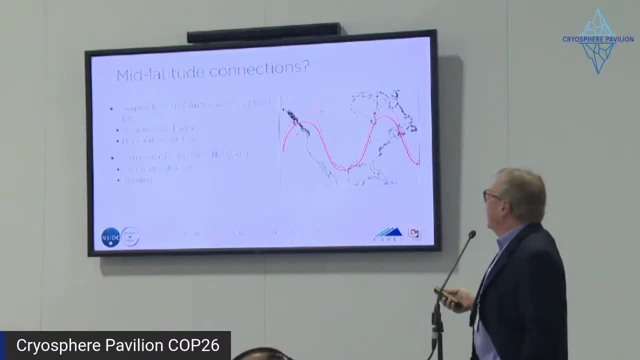 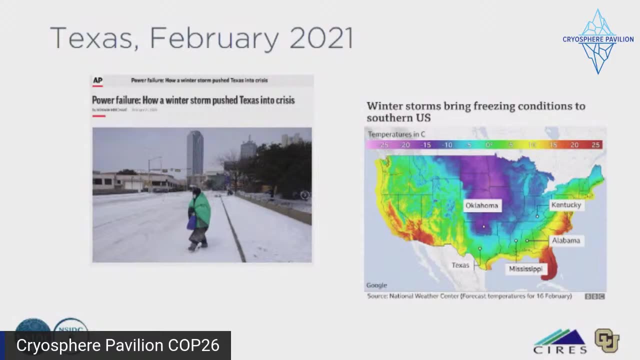 connection and, like i said, it got a lot of attention, uh, at the time, um, and it still gets a lot of attention. um, this is just this last winter. um, uh, it certainly got a lot of press in the united states. um, especially when anything happens in texas, it gets a lot of attention in the united states. um, but when they had the big uh cold. 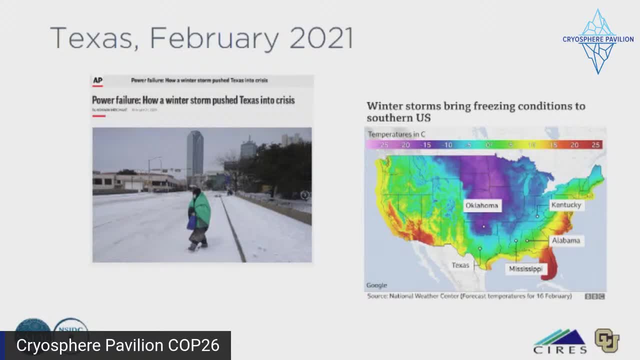 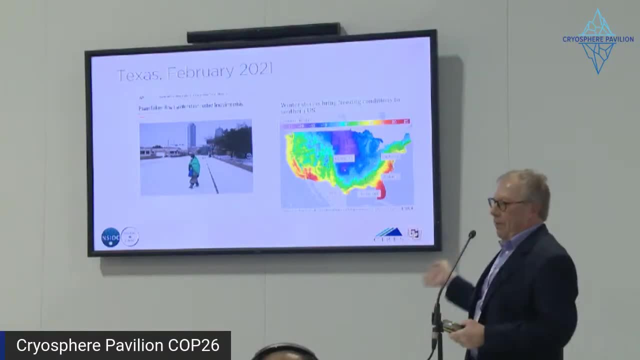 outbreak record near record low or record low. they're certainly lowest in many, many years- in february 2021, and it caused a big power failure, um, and people lost power and had pipes breaking and flooding and, uh, i think our people still recovering from that, so, um, so i had a big impact. 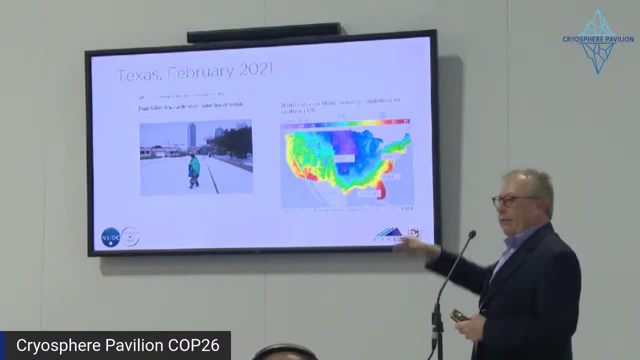 and it really, uh, you know it was a cold air outbreak, a very strong cold air outbreak. So, you know, even at this point there was the connection, or people talked about this as the warming Arctic and how that was one thing that could be contributing. 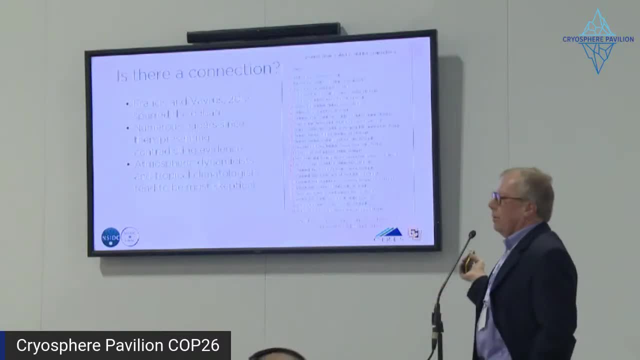 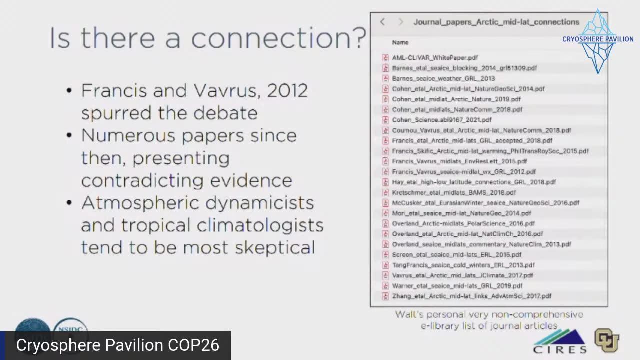 to that. So you know, is there actually a connection? So this is where you know. I think things are pretty. it's been an interesting discussion. There's been a lot of talk. This is my little. I just made a screenshot of my little library of papers I've collected And this is 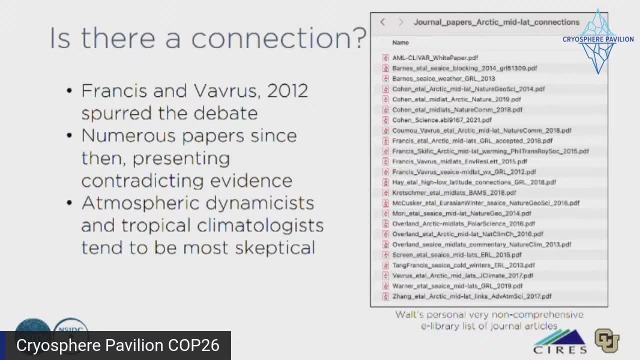 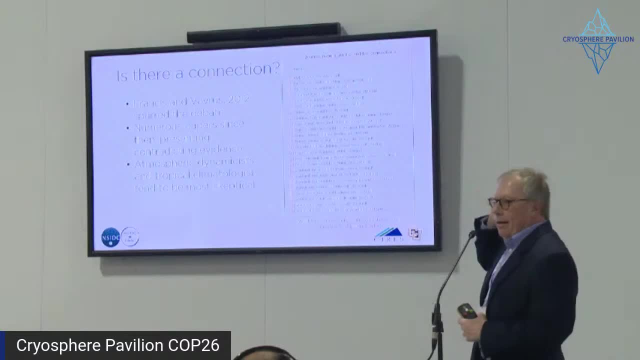 not even close to being comprehensive. These are just ones I've seen and I just save them because I think they're kind of interesting And you know there's like about 25 there in the last, you know, 10 years or so, And that again this is a pretty small sampling of them. There's a 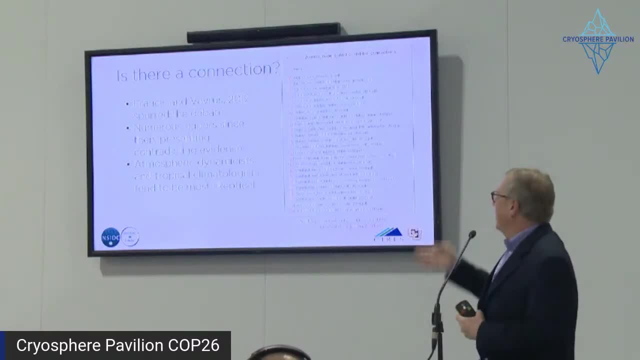 couple. I just was looking. I saw in the recent couple of days that I haven't even downloaded yet But it stirred up a lot of talk and a lot of controversy And particularly from kind of a skeptical community. there were a lot of people that really pushed back and still. 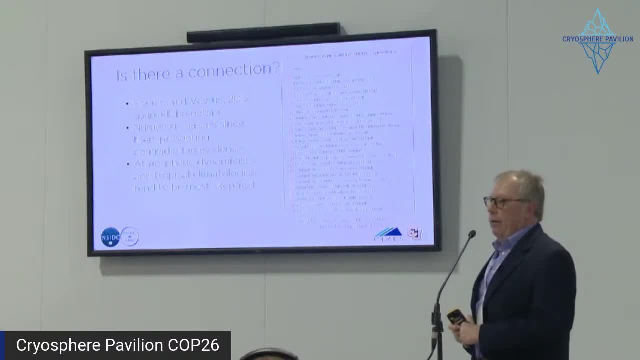 are pushing back against this, that they don't feel that there's that this connection is really there, That you know the Francis and Bavris paper looked at some data, some reanalysis data, and basically correlated these changes in the jet stream with the loss of sea ice and with the 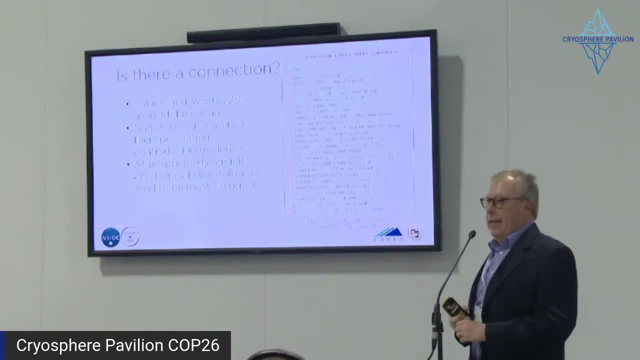 warming. And of course, we all know correlation does not mean causation And and so a lot of folks, especially tropical climatologists, atmospheric dynamics, folks that really felt that the Arctic is is is not a big enough player. It's a smaller area, There's. 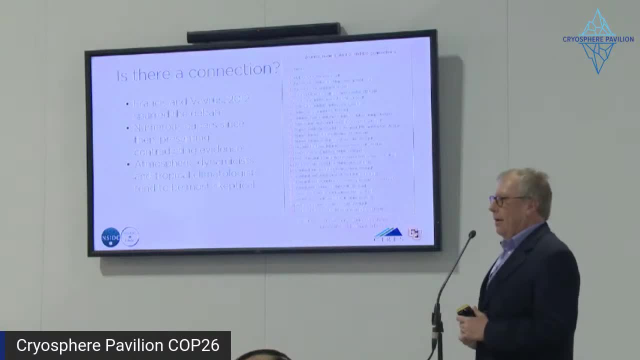 not as much energy, that the tropics are really much more of an influence on the mid latitudes compared to the, compared to the Arctic. So you know, there there was, and there there have been, several papers that you know it wasn't just. 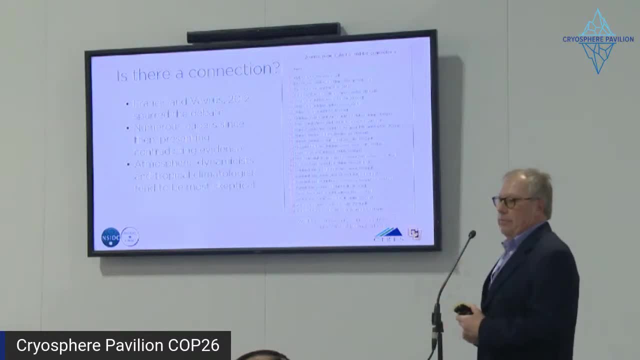 this. oh, that's you know this kind of like belief. There there was papers that have been published that showed that you know. no, there there isn't a link. They don't find a link depending on what data is looked at and how it's looked at. So it's gone back and forth. 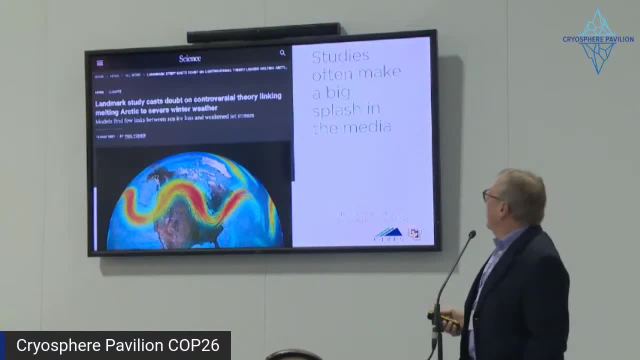 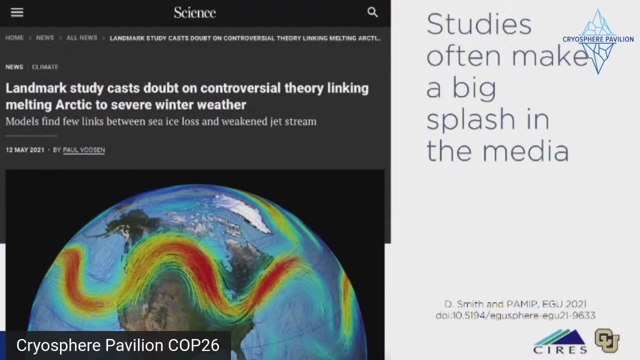 for many years. This just came out. well, I shouldn't say just came out. it came out in May and it made a pretty big splash. And that's one of the things with these kinds of studies: they, they, they tend to get a. 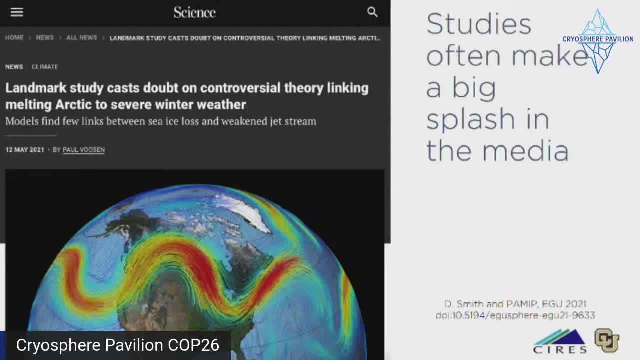 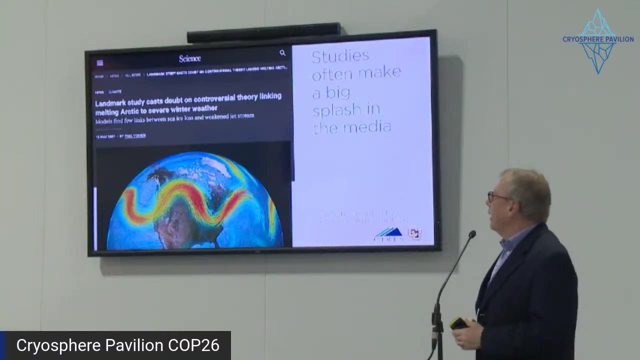 a lot, a lot of attention in the media And this one you can see from the, the headline here. you know, landmark study cast out on controversial theory. So this, this study basically said we don't find any link that it, that it doesn't. you know the the changes in the Arctic don't? 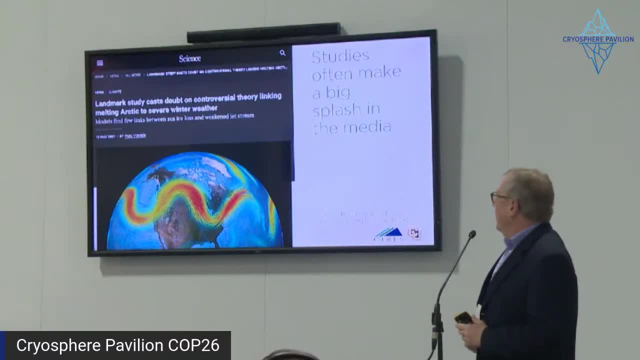 connect to that And it got played up quite a bit in the in the media as like: okay, this is it, this is the answer. This is you know, we we've got it. there is no link. You know that that. 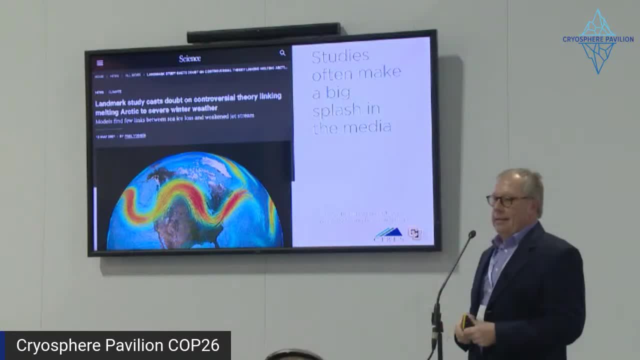 that headline and this is even. this isn't science, So it's not like this isn't, you know, a tabloid New York Post or whatever. So but the thing that that is interesting here is this is: this was a a presentation at the European Geophysical Union. This is not a. 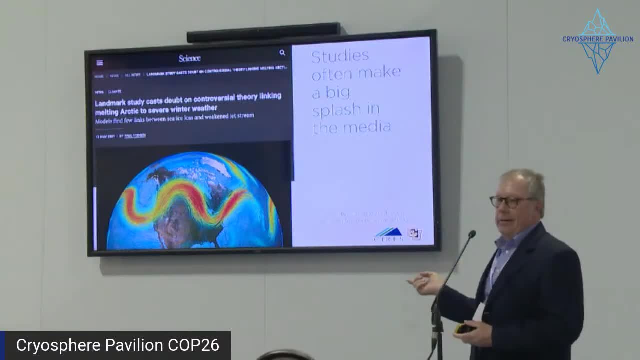 peer-reviewed paper. I assume they're probably going to publish a peer-reviewed paper. I haven't seen it yet. But you know, this is just a a, a small talk at EGU. you know this, that's generally research in progress And, yeah, it's still got a lot of attention. 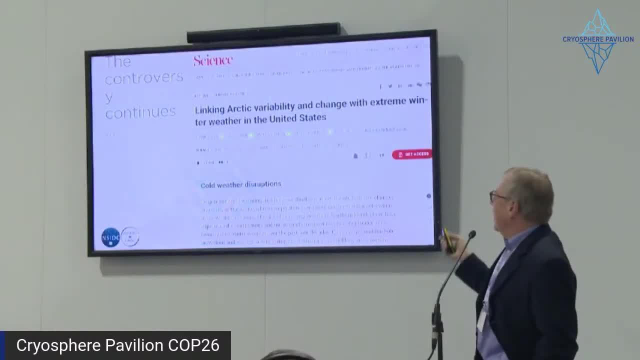 And then you know, but nonetheless this just came out in September. Judah Cohen's one of the folks that have been pretty big into the research and have have found some links between the variability and extreme, especially in extreme winters. So this was in September. 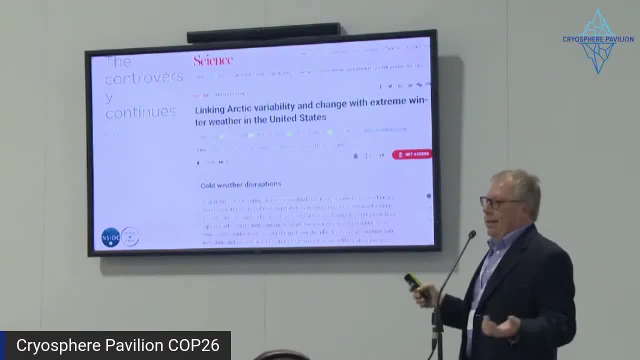 and saying, yes, there is a link, So it- you know it- really gets into the weeds. There was a big National Academies, US National Academies study on this and workshop on this way back in 2013 or 2014,, I think it was, And you know that was. a big report came out of that. But even since 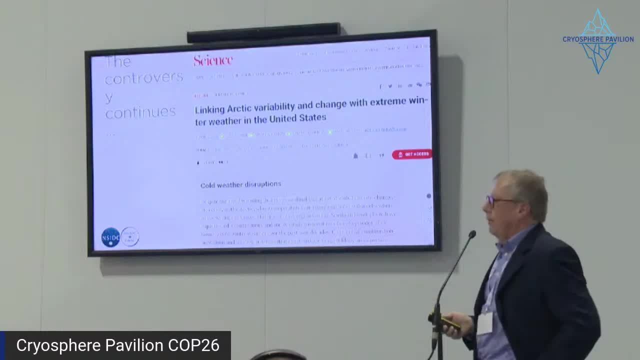 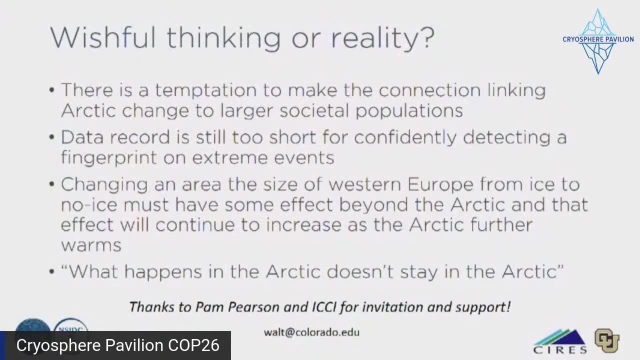 then I think we're still in this area of you know, we don't really know, And and you know, I think one of the things that's it's a concern is it may be wishful thinking to some degree. 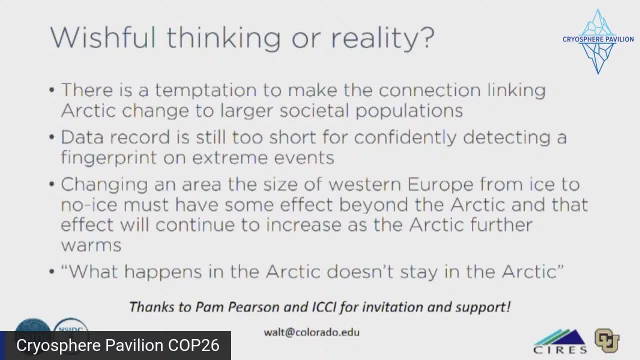 Not to say that, like Jennifer Francis and Steve Bavris and others that have found links, that they're they're making things up or that they're they're not interpreting the data correctly. I mean, they're really great scientists, You know. I know Jennifer and Steve and they do. 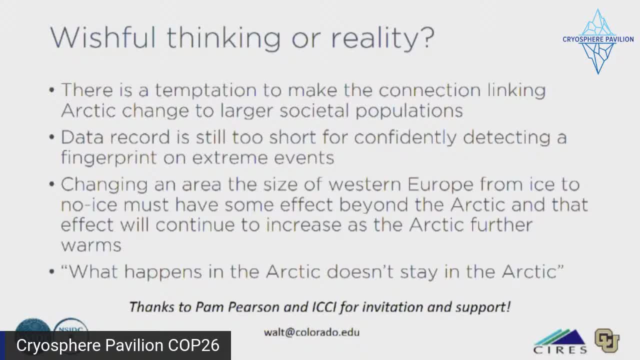 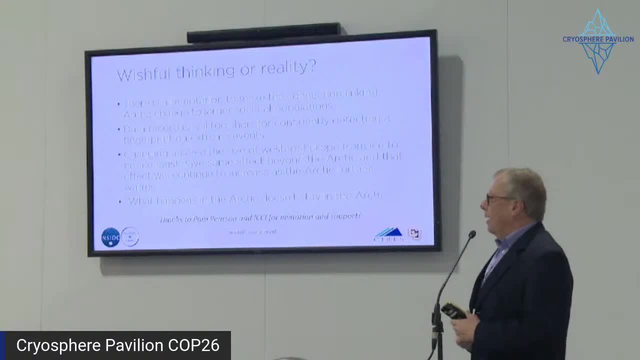 great work and their- you know their- papers are good, but I think there there are things that you know, depending on again when, depending on how you look at the data. it's hard you can come up with different answers, And one of the things is we're looking at extreme. 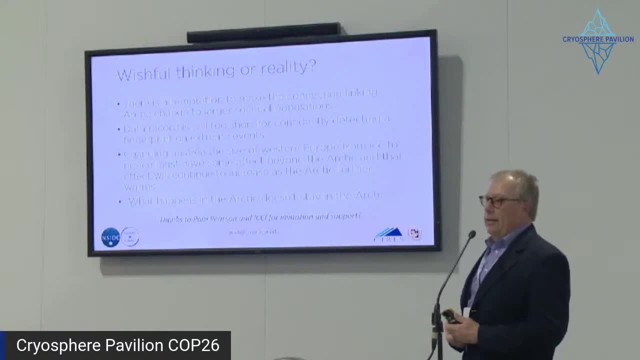 events and extreme events are, by their nature, rare, And trying to detect a signal in extreme events and a record that's only about 40 years old is very difficult to do If you've got something that happens only once in a century and it starts. 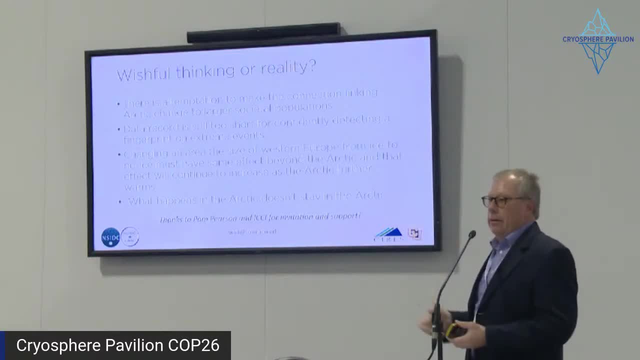 to happen and you've changed things. So now it happens once every 50 years. Well, do you actually see that in a 40 year record? You know, there are other ways to do, you know to do kind of attribution and so forth And and people have started to do that, But it's still, I think, too. 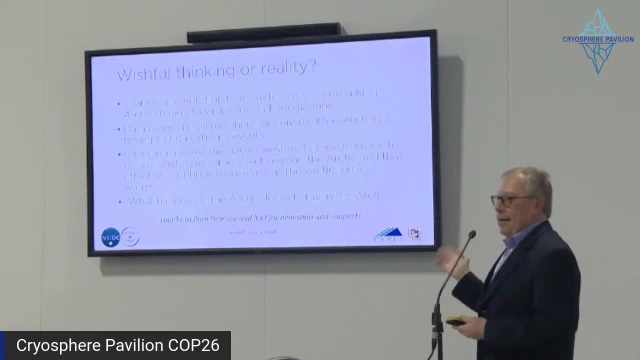 short to really detect it. And again there's this temptation, I think, to, in wishful thinking, to try to make that connection And as a scientist, I think we have to always be careful about that. You know one of the questions, as someone who works in the Arctic give presentations. 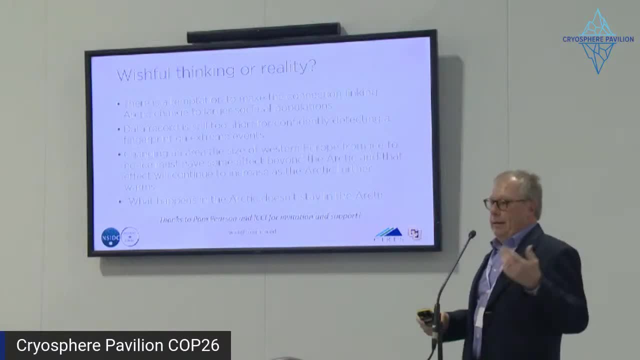 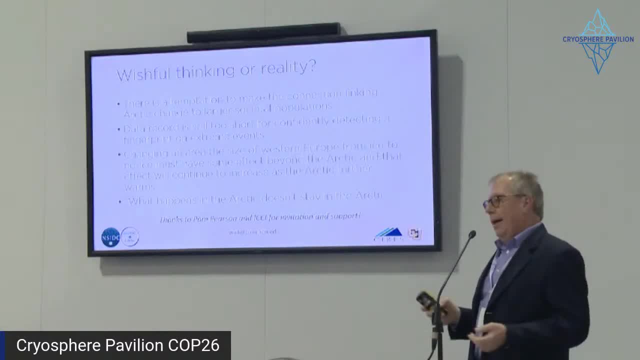 that's how itiens an Arctic ice sheet. So the loss that's like the opposite of what you know For Greenland and радica ice sheet, sea rise. you can make the connection for sea ice. It can be hard to do. you know you can talk about how sea ice is. a is a bellwether You. 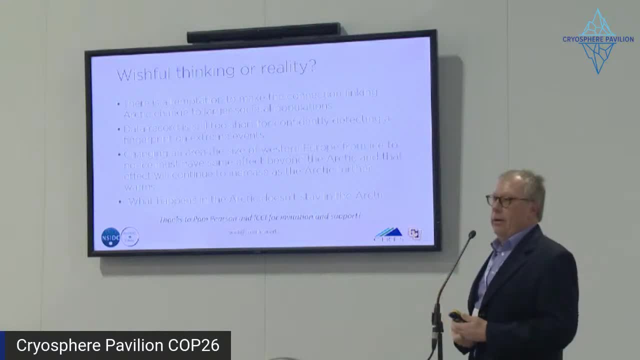 know the changes that are happening with sea ice are going to happen to the rest of the globe later, But there's that temptation and desire to really want to say no, the sea ice loss is going to affect you directly And so this is this mid latitude. 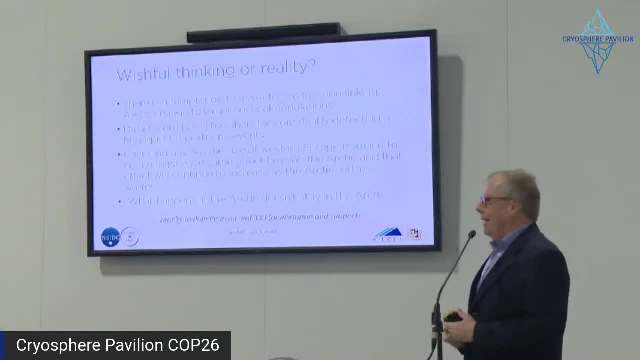 teleconnection is a great thing to to make that connection, to say that big snow storm you you had, or that big heat wave that was due to the sea ice, or partly due to the sea ice, um, or the arctic warming, um. but you know, it's hard to say if that data is really there yet, but i i caveat that also. 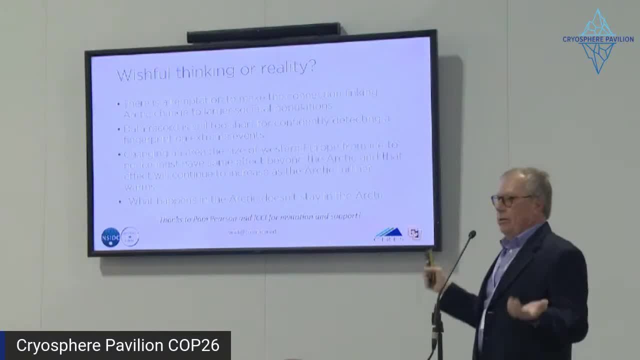 with. you know you're taking an area roughly the size of western europe um the arctic ocean and you're changing it from almost completely ice covered year round to being almost seasonally ice free um during, at least during the summer time. you know that's changing the albedo from. 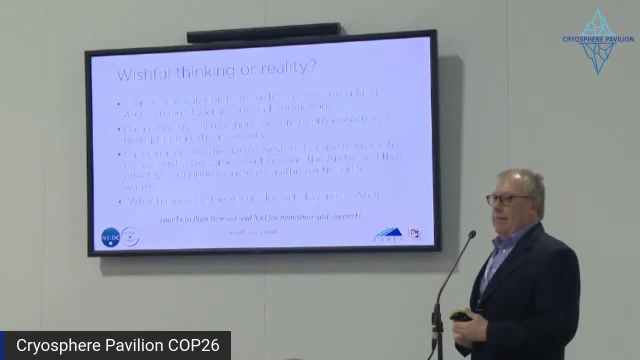 you know, 0.7.8 to 0.1 um, that's a huge change over a big area. um, and i, you know, i just don't think you can make that big of a change without having some effect outside of the arctic, um, and 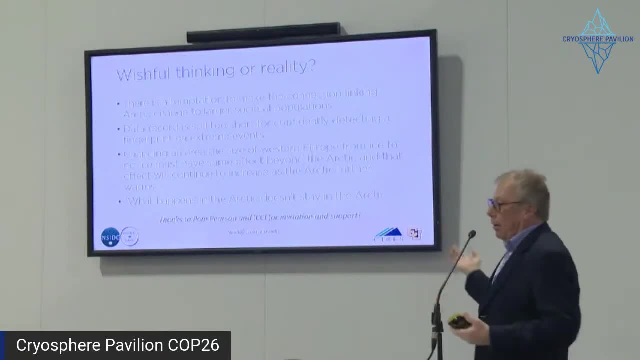 i think as that, as the changes continue to occur and as we get a longer record, i i think we will start to see um some signal outside of the noise, um, and you know, the, the sea, ice is changing, um, and so something's going to be happening. that's going to be happening. 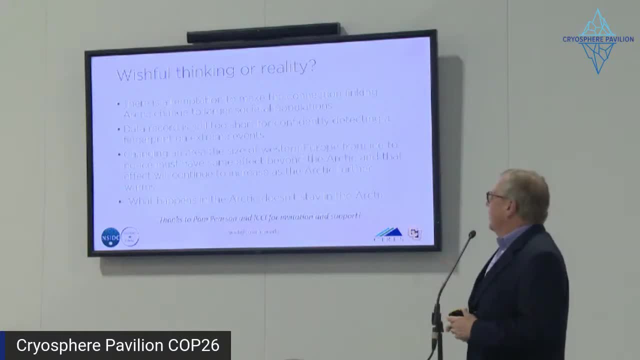 later. but, um, i do think that the arctic is changeable. it's changing the atmosphere, it's changing the climate, and i think that's what's going to be happening in the arctic. so, uh, also, uh- i- i think this has been mentioned many times before- what happens. 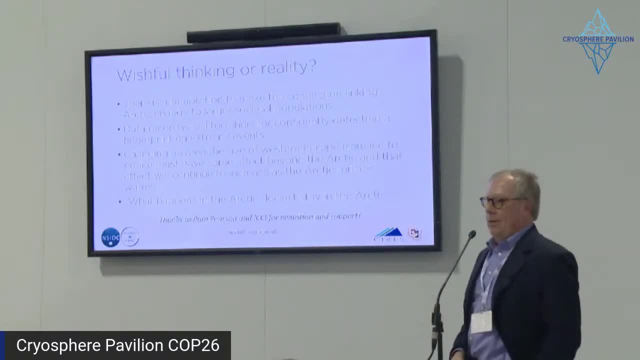 in the arctic doesn't stay in the arctic. i do think that that is true, and so so i think i'll end it here. i want to thank pam pearson and the international crisis, your climate initiative. you very much, waltz. um, i want to know, does anyone have any questions online or on the? 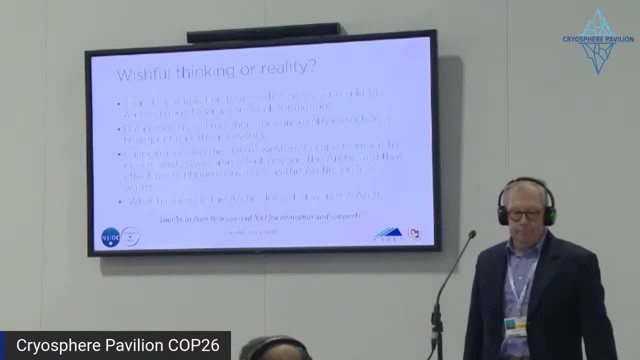 floor. does anyone have any questions for wolves? sorry, i've got a very quick question. with regard to the definition for extreme events, how can we define them in a way that would not cause questions and concerns from climate dinars, specifically, because, yeah, that's something that they use a lot. yeah, um, very good question, and i didn't actually define extreme events, um. 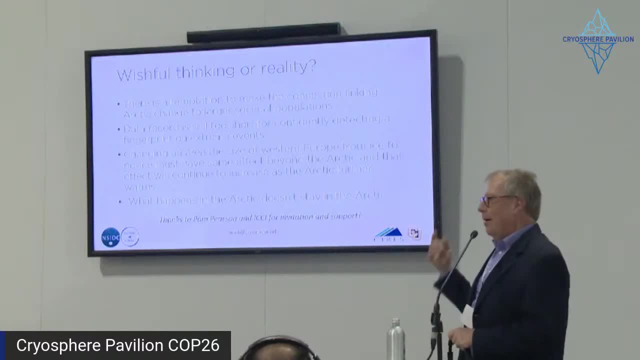 because you know it's, i think, in a lot of ways, and like it's talked about, uh, in terms of, you know, extreme being something that has a big impact, that's rare. um, you know you could use statistics, uh, you know, uh, something that's a three sigma event would be an extreme event. um, for example. um, 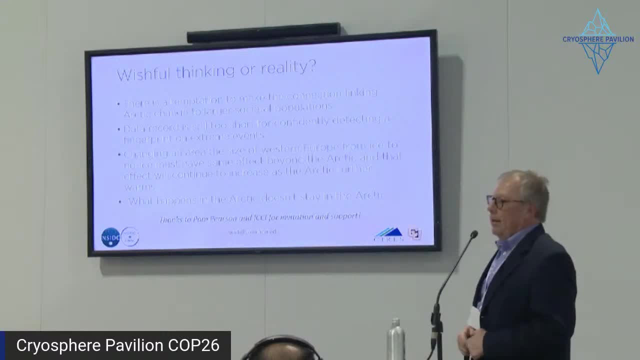 or or even hot, you know even higher um. so that would be one way to define it, using a, a base period um, you know, storm frequencies or something like that, and looking at the uh, the deviation from that, if you start getting you know out of beyond three sigma, that's something that seems you know. 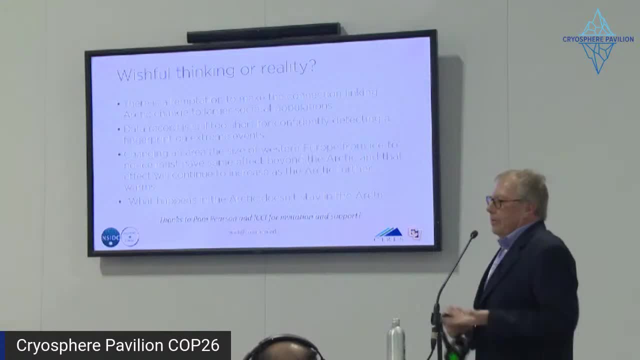 really rare that that's outside. or even two sigma you could consider. two sigma is kind of the you know the 95 range, so that would you'd be in the five percent um range, so that's one way of it. um, i'm sure people have have uh specific ways of yeah, i mean, i know that people have specific. 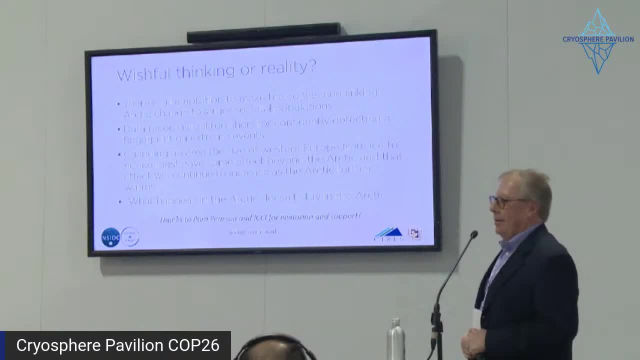 ways of doing it, but i i here. i didn't define it specifically, um, but i think that's a good point. definitely, yeah, so thank you very much for the presentation. so you wrote there. the data record is still too short, and so my question is: may paleoclimate studies from ice course uh can help in bridging? 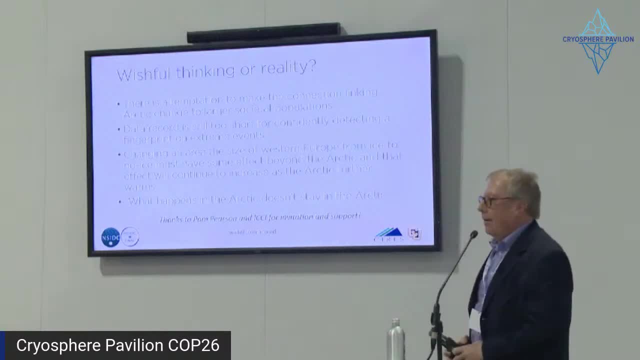 the knowledge gap. thanks, yeah, great great comment on that. um, and definitely, i mean that's the paleo climate record. um could certainly help. um, you know i i'm not a paleoclimate person at all, so yeah, i'm not sure what kind of events might get captured in that um. uh, you know things like 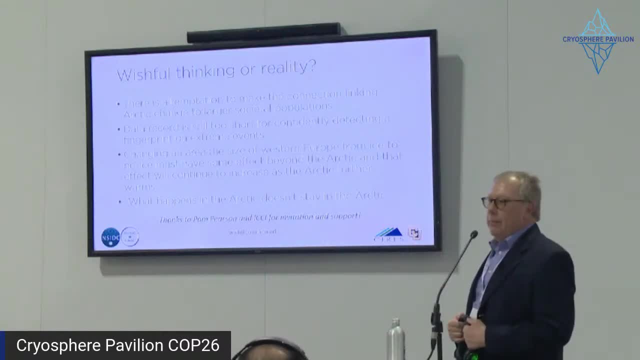 coastal flooding and things like that. potentially could i think um, but i think, yeah, that's a resource that we could certainly look at. um, and probably people have looked at that. you may be more familiar with that, but um, yeah, um, i think that's a good point, yeah, so i actually have a question, but oh, 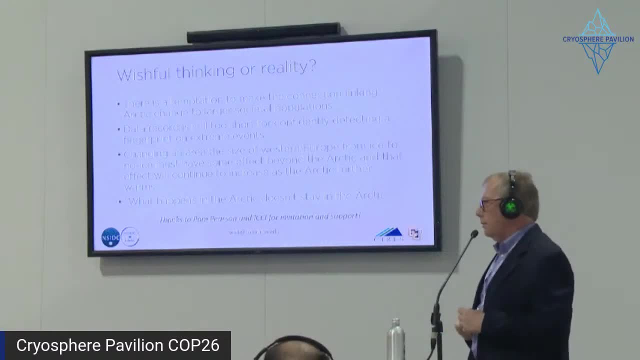 we've got some more questions, well, so one thing i was just wondering about just off the back of that question was, uh, the resolution of the data that you're you've been using to uh to look at these um effects. i assume it's fairly coarse resolution to cover the whole of the arctic and 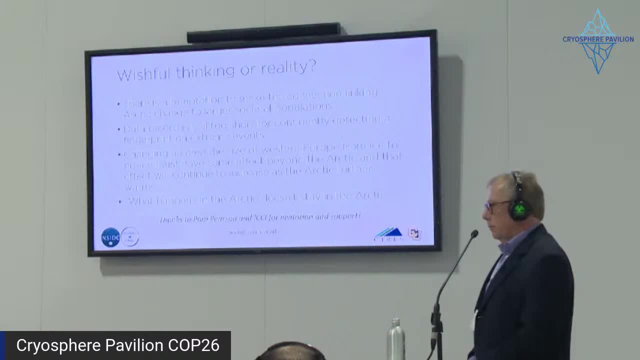 i was just wondering, as, as techniques get more and more advanced and we're able to simulate down to a higher and higher resolution, maybe pick up some, um, high resolution convection, for example, do you think that? uh, the amount of extreme weather events that we pick up and the frequency, do you think it? 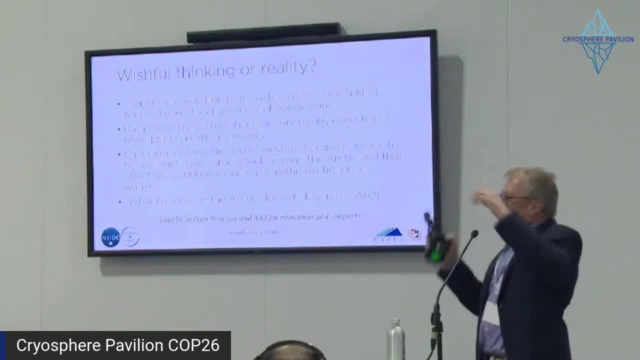 will change in these studies? yeah, good question. um, yeah, it certainly. it certainly could. i mean, the reanalysis data that's used for the atmospheric um variables is, uh, like, basically one degree and and of course, the thing there is that you know it's reanalysis is using models. 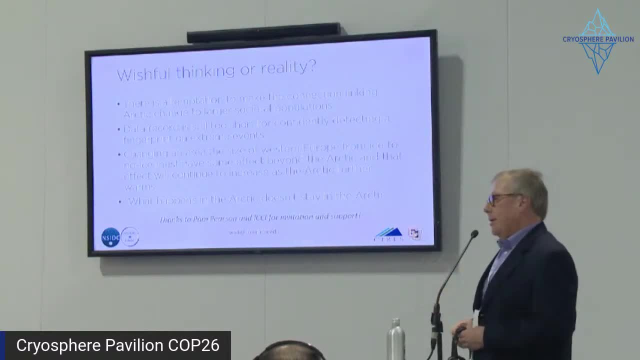 and integrating in observations, and in the arctic observations tend to be. it tends to be fairly, uh, sparse in terms of observations, particularly over the arctic ocean. um, especially, you get anywhere before, like 1979 or so, um, before. yeah, there's been buoys since then that fill in some of the arctic. 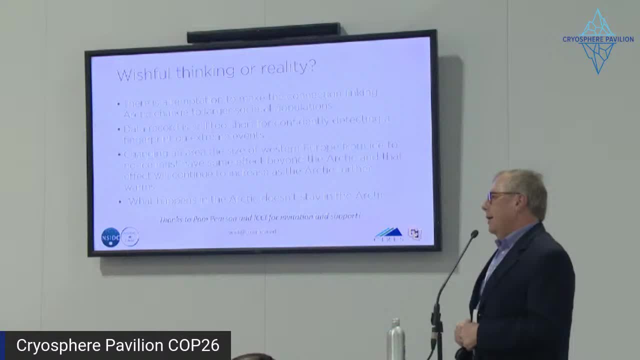 um, and there's been more coastal stations, um, so, yeah, you have a pretty coarse, um, you know, set of data that's going into that and you're not going to capture some of these smaller events, um, that that, uh, that can occur, and so i think, yeah, if you, if we get to better data, finer data, 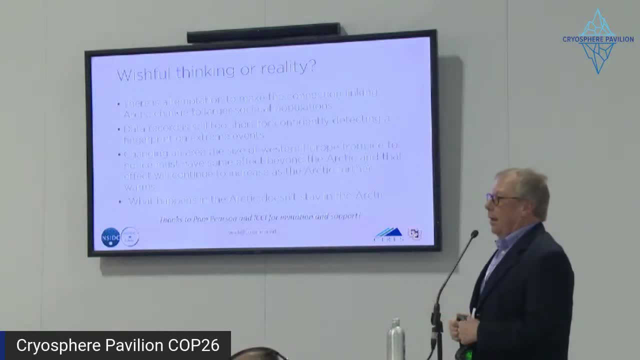 you know where we. we have more data and then finer scale modeling. um, you know the models are getting uh, higher resolution. um sea ice models- we can get down to 10 kilometers for some some models. um, so that's starting to get some some small scale effect. 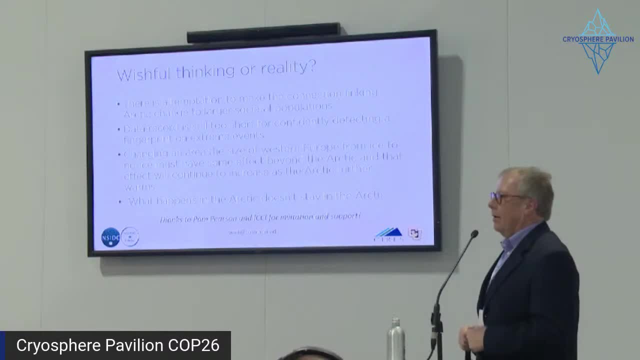 but that's certainly a a limitation, um, in terms of our records. yeah, i think there's two more questions. thank you all for a very nice presentation, a highly interesting presentation. uh, roll throne from amap and your- i mean your- conclusion kind of reached the same as we do. 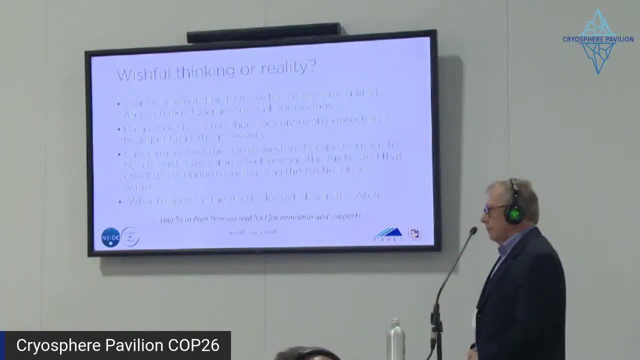 in this our latest report on the teleconnection chapter um, and i think how you ended it here, talking about picking up like an extreme signal um by retrospective data is impossible, as you say um. but i was wondering and we'd like to just to speculate a bit like if, if we kind of 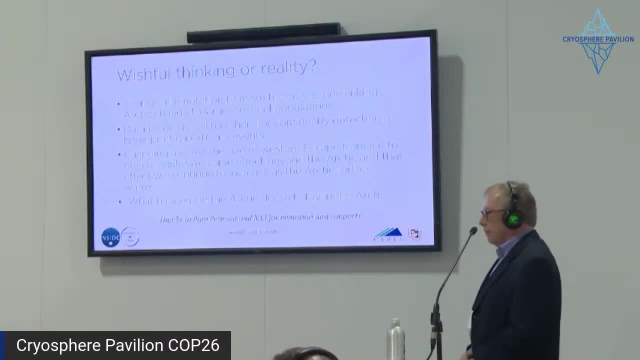 agree upon we. it's very hard to pick up a signal of an extreme event or like a change in extreme events because, due to the their nature, would it be any other part of the processes or mechanisms? when it comes to this sea, ice, uh, air, fluxes of energy and and possible talent connections, are there any mechanisms or? 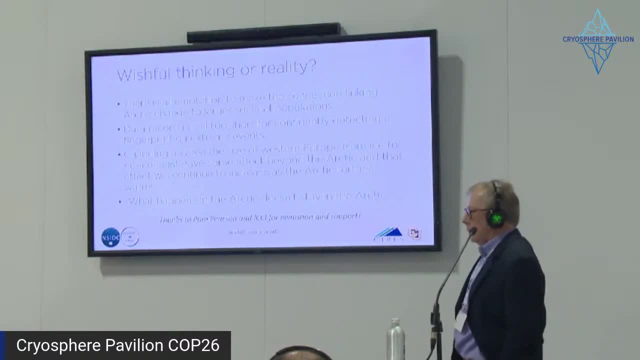 or processes that are particularly good candidates to look into to try to find this kind of connectedness between arctic and low latitudes? yeah, good question. um, uh, i'm not probably the best person to answer that, because You know someone like Jennifer Francis would be a really good person to answer this or others. 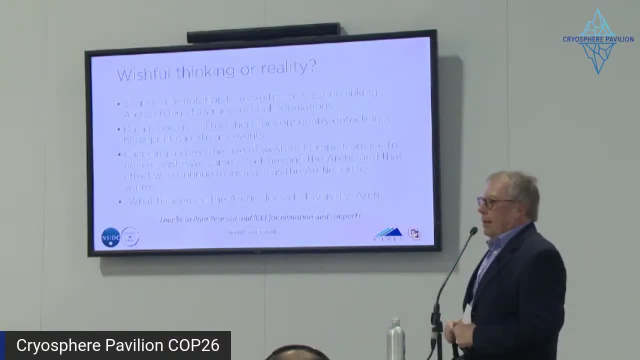 But the- Yeah, you know what they looked at was this: you know kind of the waviness of the jet stream and how far the jet stream goes north And and you know one of the things is that you have these rare events happen. 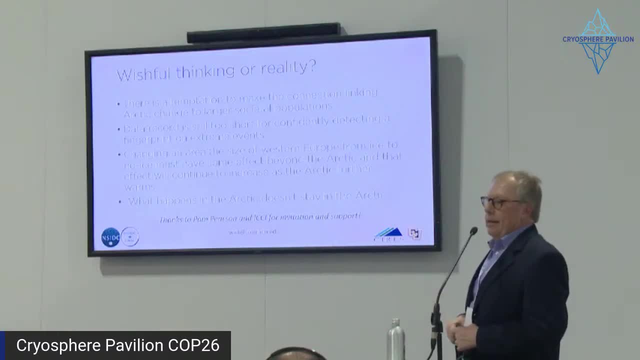 You know nothing, far as I would say- not that I have seen- nothing unprecedented has happened, So it's just a matter of frequency. So that lends the idea that you just need more and more data. But you know the physical mechanisms. I think it's the thing that that people have been connect. 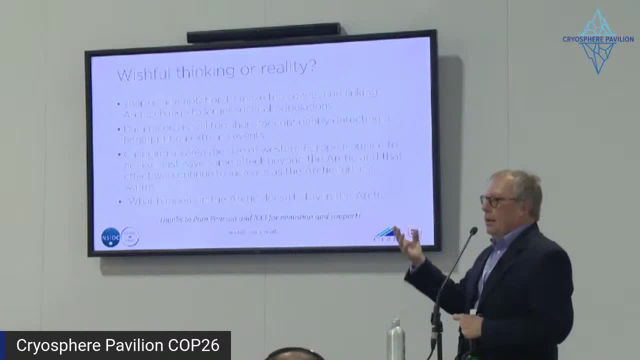 You know you have warming in the, in the, in the Arctic. that warming, you know that warming starts to go up. It helps spin up the stratosphere. The stratosphere can break down and then the stratosphere connects with the troposphere. 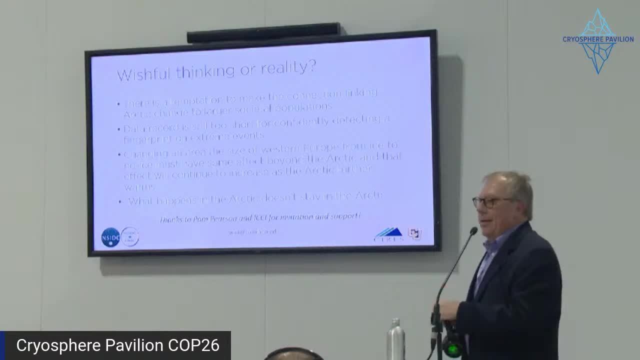 And that's what kind of that's? that may not be a very coherent understanding, of the top of my head, of the Connections there, But you know. so there have been some of these physical mechanisms that have been theorized and looked at with models. 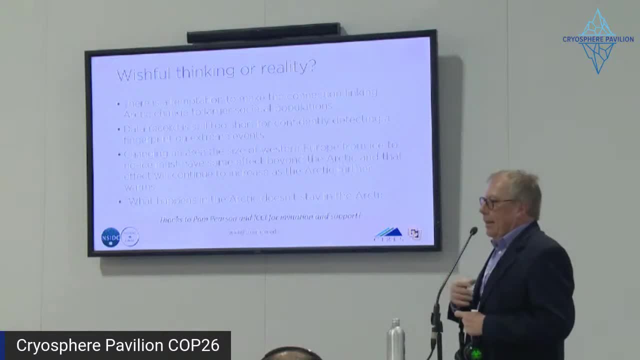 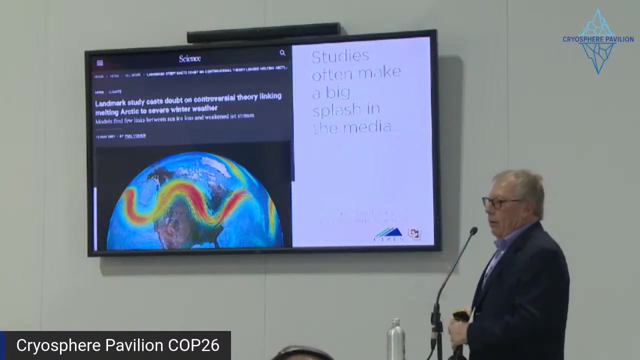 And this is where I think it, it gets interesting and certainly out of beyond my real understanding. at least easy understanding is: you know, you get into the modeling things And you know this paper, you know this landmark study did like it was a model and they, they said: yeah, hey, we did it with lower sea ice, with higher sea ice. 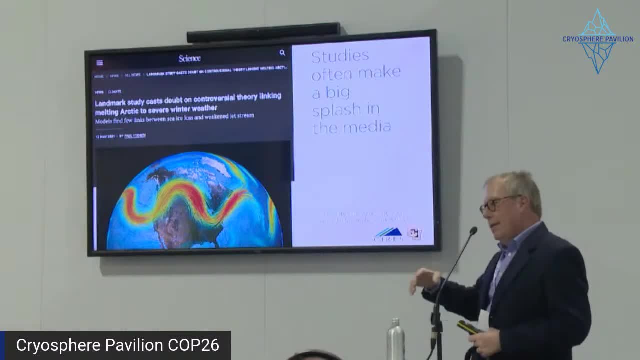 We didn't see a connection. But does the model Have the proper physics to make that connection? You know again, I don't. I'm not a modeler, so it's hard for me to really evaluate that. Other models, though, have other modeling studies have shown. 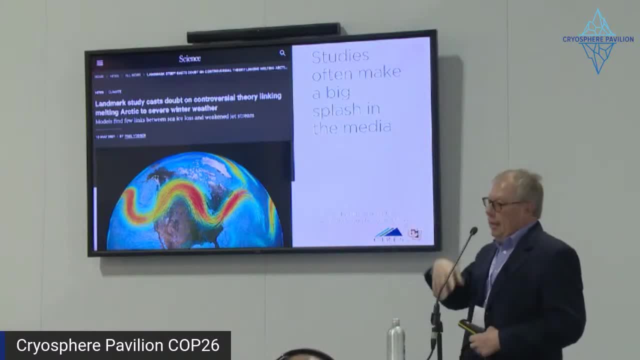 Yeah, we do it this year. We run it with less sea ice and we do see increased storms and you know, in China or northern Europe, And that's the other thing that I think is as difficult about these. You get these extreme events. They happen in different places at different times. So that makes it even. it's not like You know, every October storms are becoming more frequent, or something like that in northern Europe. It's like you know, one year it's you get a really cold outbreak in the eastern US. 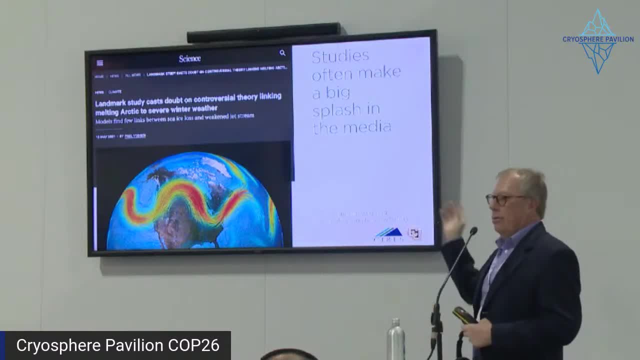 The other year it's in northern Europe, The next year it might be, or two years later it's in China or in you know. so it's. it gets really hard. So I think, making better physical connection between you know the actual Arctic warming and you know the troposphere, the stratosphere and the connection with the mid latitudes, 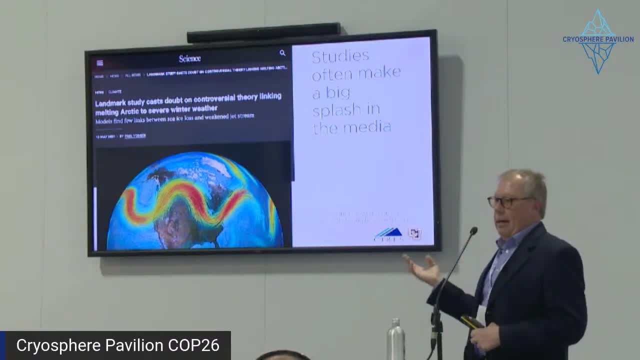 And getting models that that I guess we have more confidence in. or, you know, maybe higher resolution that gets the more fine scale physics that we can, we can compare. I think maybe that's the the the answer ultimately, to try to do that along with more data. you know that we can start to see a signal outside of the noise. 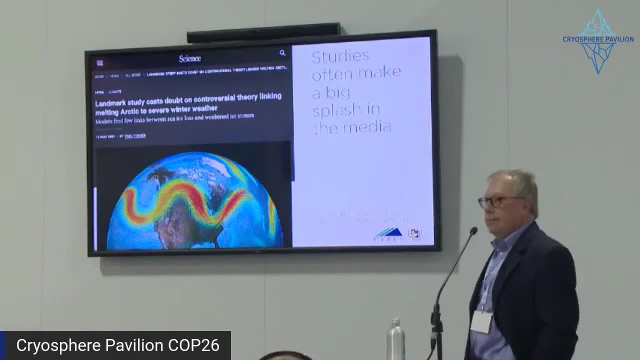 So yeah, Are there any more questions? Do you have a question? Thanks, you'll have to indulge me for a second as a complete non specialist. So just to understand, unpack a little bit. So this paper or this presentation was saying that's, that's not the cause. 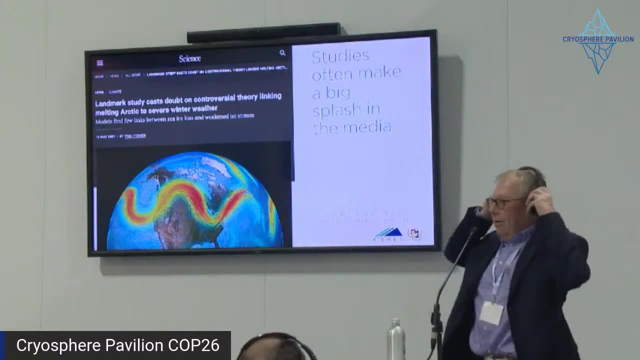 What is it saying is the cause? Yeah, good question. I don't remember the specifics right off the top of my head right now, but if I remember correctly it was the tropics that they saw. I think it was Pacific changes in the Pacific circulation. 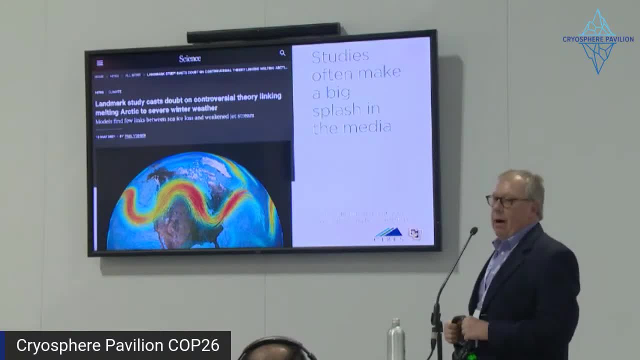 In the North Pacific, I think, particularly where they were, the driving mechanisms. Yeah, yeah, that's a good point. I mean, if you, if you're going to say this isn't the cause, something else has to be the cause, or should be right. 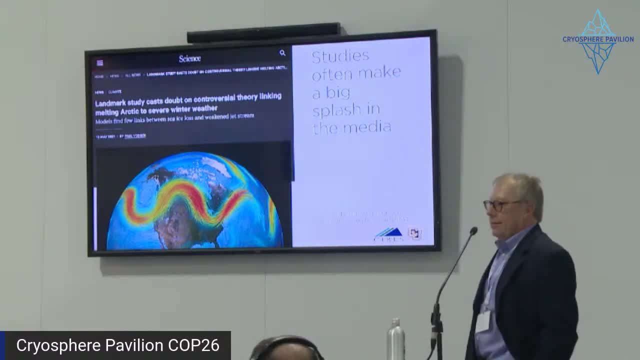 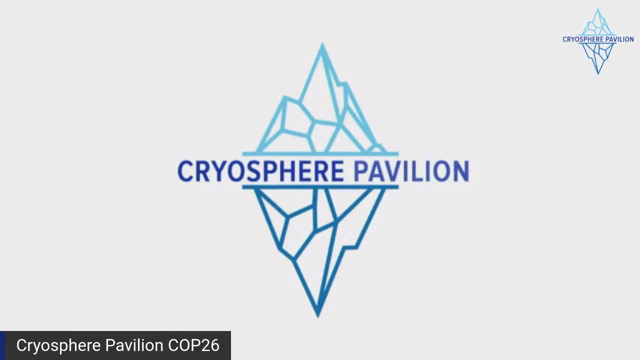 So they did talk about that. Yeah, OK, so I want you to join me in thanking Walt again. Thank you very much. Thank you, Thank you.